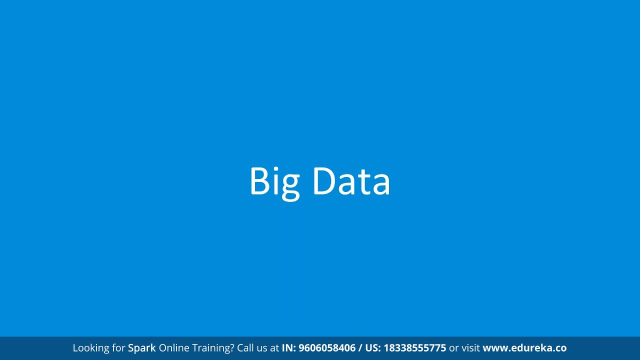 electronic gadget. No right, What you would say? you would say that Sunita, this came into the market long back. That time requirement was different. So over the years, everything has changed. So today you'll say that, okay, we need something which is designed specifically for today's need, As in. 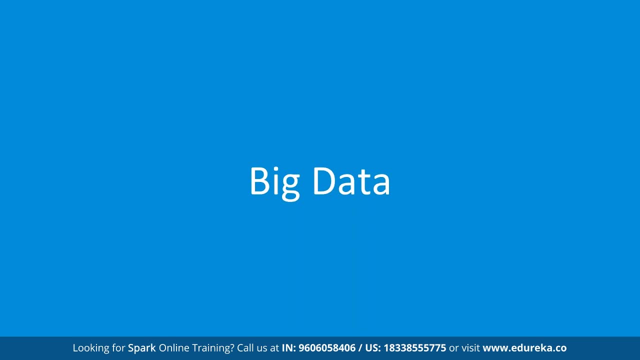 these days we are using smartphones. If someone is asking you to use landlines, you would feel a little bit uncomfortable, Because now you know that technology has. you know, technology has evolved and our needs or requirement has changed and smartphone is helping us out in n number of ways. Okay, So now. same is the scenario with big data. 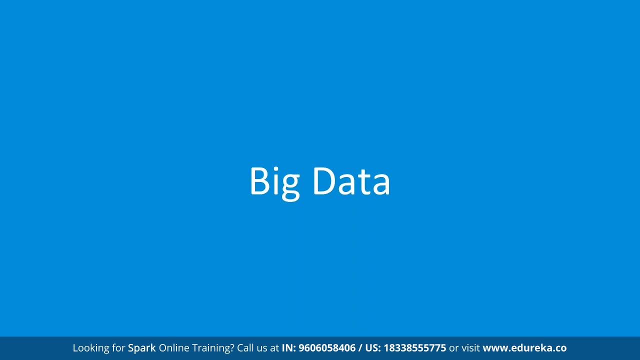 So, first of all, what is the difference between data and big data? Data is usually small amount of structured data, as in 20 to 25 years back, we all were not generating huge amount of data, right? We all were not involved in It's like we were. we all were not involved in generating the data. 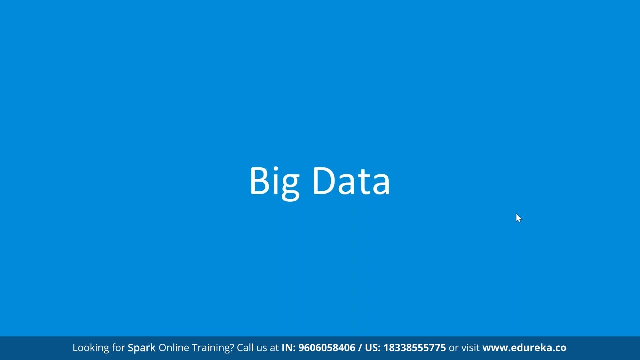 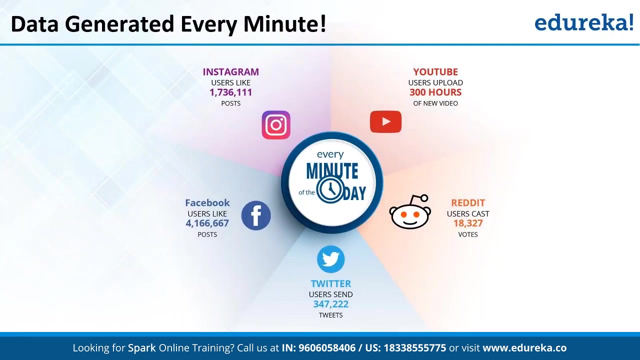 right, We were not dealing with electronic data as much as we are dealing today, right? So over the years, like we have moved from data to big data. So what is this Big data? technically, Yes, So this is big data, as in, data is getting generated every minute. 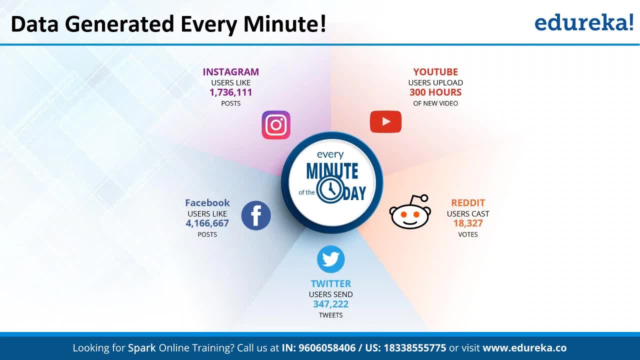 So, if I take example of social media platforms, right? So? it's like on YouTube, every minute, 300 hours of video is getting uploaded: Instagram, these many likes, Facebook, Reddit. So what is it? It's like data is getting generated every minute, Plus, it is not only the structured data. structured. 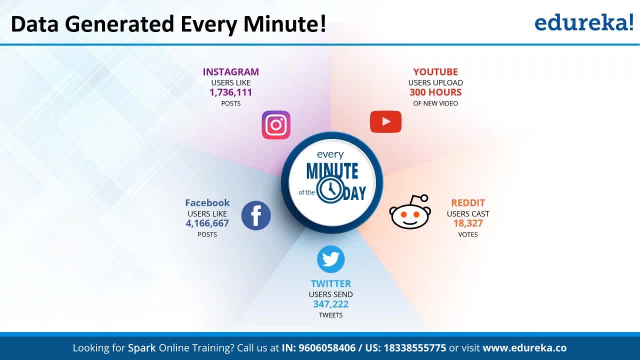 data, as in which can be stored in form of rows and columns, But when we talk about the data which we have on the social media platforms, it's, it's. it has got every kind of data and it has got structured It. 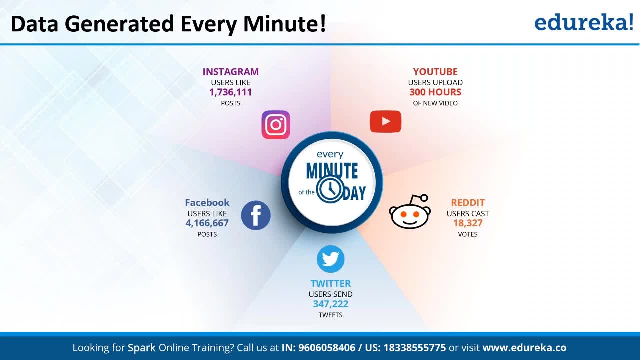 has an audio video, text images, right. So now, if I tell you that, Hey, we need to process this image or we need to process this video, do you think you'll be able to use our DBMS, which came into the market 25 years back? No right, You'll say that the purpose of our DBMS was different. Our 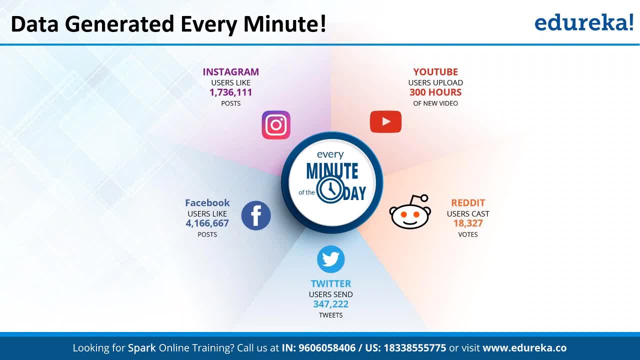 DBMS was designed specifically for structure data. So now, in order to process this audio, video or image data, right, We'll say that we need a different tool or a technology, right? So that's why we say that big data is nothing, but it's a problem which industry is facing right now, as an industry has got 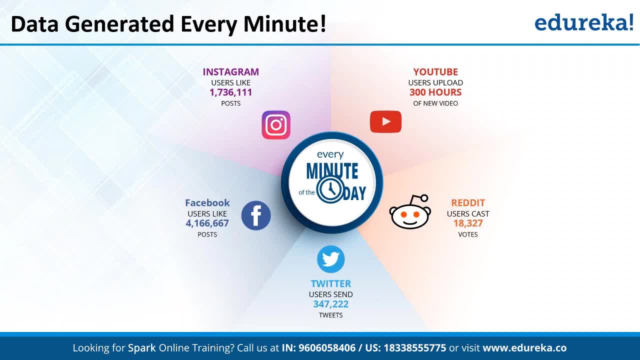 resources. who has got expertise on legacy system or the traditional system? right. But that expertise is not going to help us. Doesn't matter If you have On our DBMS, let's say for 10 to 15 years, that will not help you here, right, Because the purpose 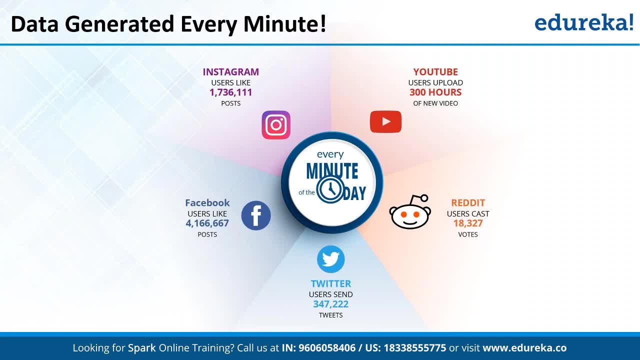 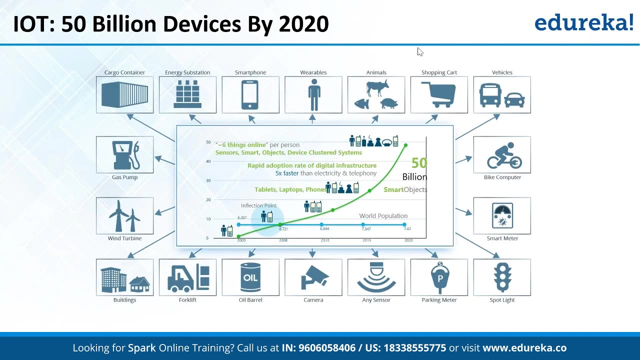 of our DBMS was different, And now the requirement has entirely changed, right? So that's why I've got industry saying. industry is saying that it's a problem. We don't know how to store it, how to process it or or how to do the analysis on it. Okay, So now? um, it's like data is increasing. 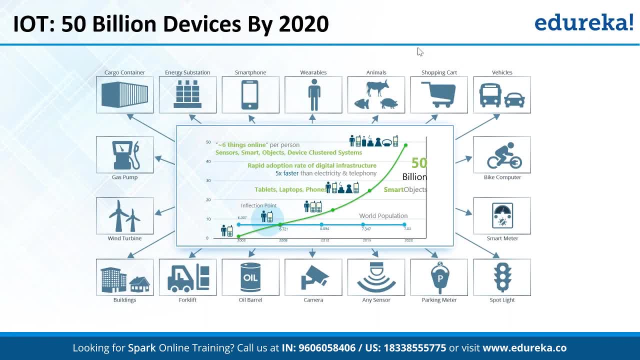 like anything. even you all know, right That, uh, we, we are using a number of smart devices today And and every device is generating the data and everything is happening in real time, as in right. It's like if you have ordered food from the matters, you can track it real time. 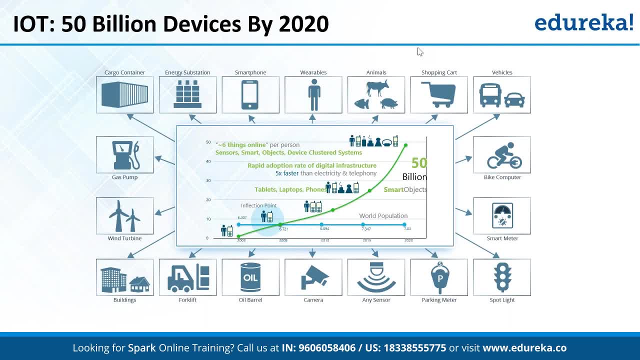 or it's like we have uh uh fitness devices, right Fitness trackers, And there also we can track it in real time. So everything is in the data right. IoT is nothing but internet of things, as in where we are connecting the devices or the sensors to the internet and data is getting. 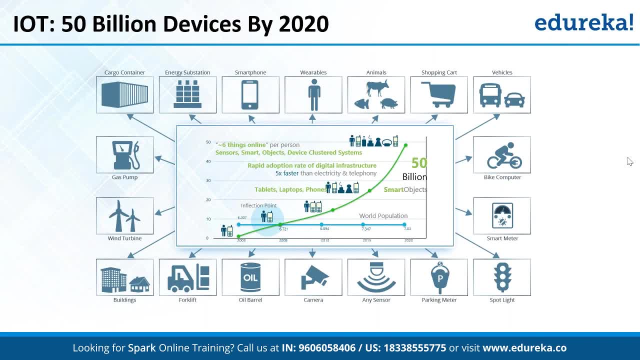 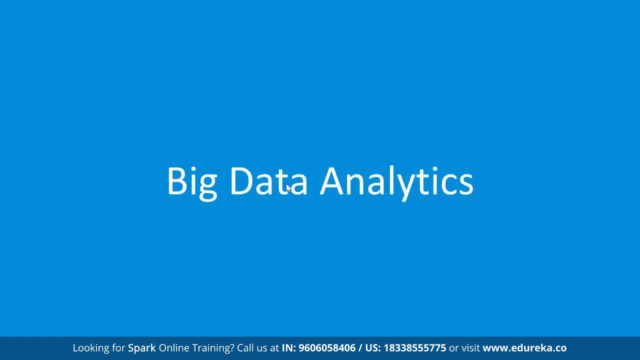 generated continuously For the analysis purpose, So that analysis can be done in real time. Okay, So now big data analytics- okay, big data, It's just a term which means use amount of data getting generated at a very high speed And also which has got varieties of data, And this is how data is- is different from big data. 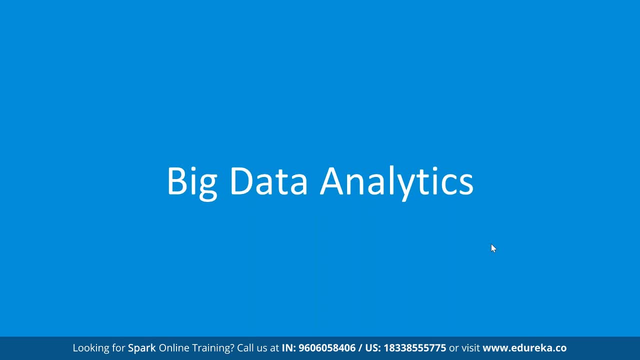 Fine, So now big data: analytics, as in. you will be doing the analysis on this huge amount of data which is getting generated, generated continuously and which is having varieties of data, so it doesn't matter if it is video data or if it is audio data or text data. you will store it and you will do the analysis on. 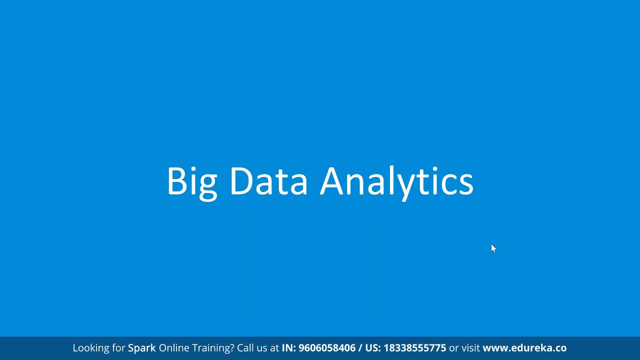 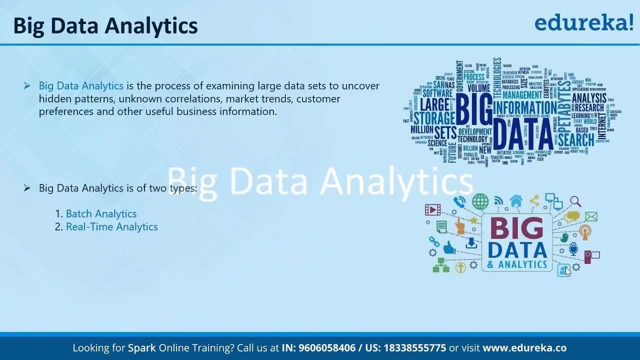 that right. so now the purpose is why we are interested in doing the analysis on this data. so basically, big data analytics means doing the analysis on huge amount of data so that we are able to generate more accurate reports. okay, i will take one example here, as in in my class. 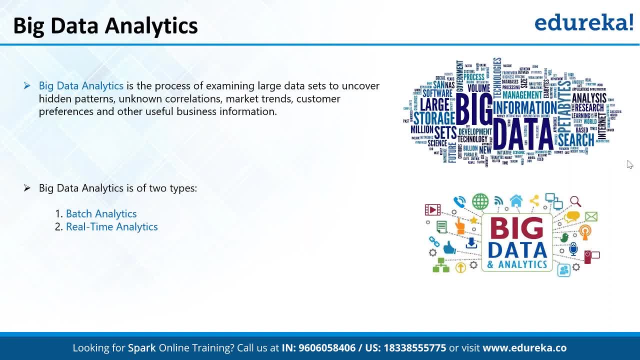 there are tens of rahul. okay, in my class there are tens of rahul and i want to talk to a candidate name rahul sharma. so what am i doing? i am just calling out the name rahul. so do you think that? 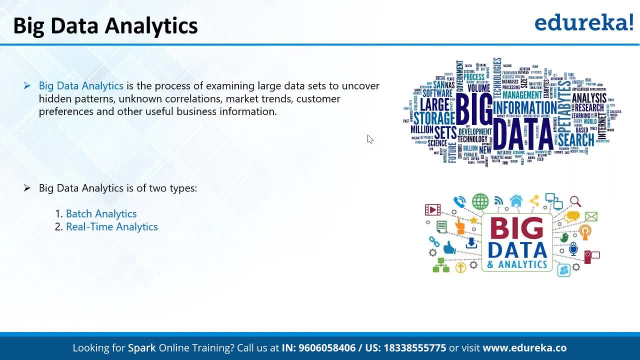 i'll be able to the i'll be able to talk to the right candidate. no, right. so point is, if i use, which is nothing but extra data, i'll be able to talk to the right candidate, as in more the data we have, more accurate reports we. 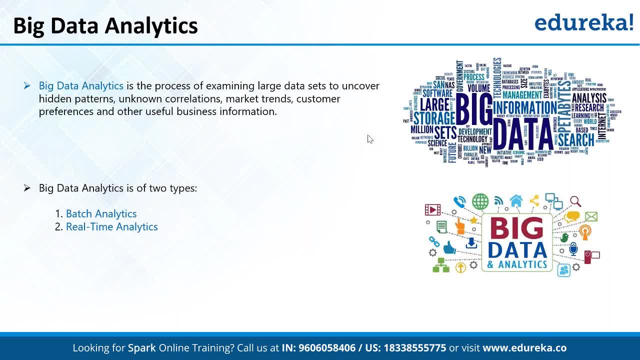 will be generating right. so big data analytics? eventually, the end goal or the objective of big data analytics is to keep the customers happy, right to generate more accurate reports, to find, like the hidden patterns, correlations, what is a market trend, what is a customer preference and other useful business information. okay, 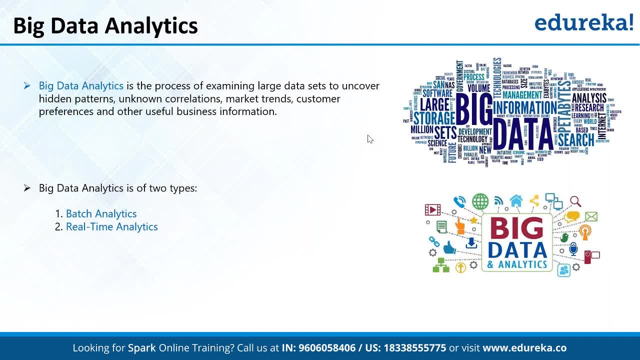 you so you can take example of any domain i already took. it's like i i already i already took example of you know healthcare domain, like where we, where i said that, okay, we do have like in i watch, right, there is a feature. so it's like whenever the heartbeat is is going low, the notification will. 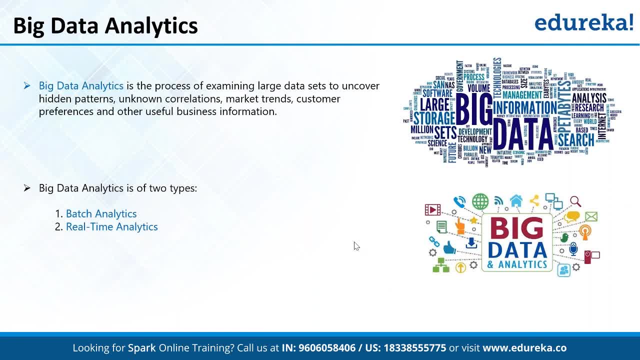 be sent immediately to the doctor. so what is that? it's like analysis on the data is being done continuously and it's happening real time, and it's like the purpose is to generate more accurate reports so that we can be able to generate more accurate reports, so that we can be able to generate 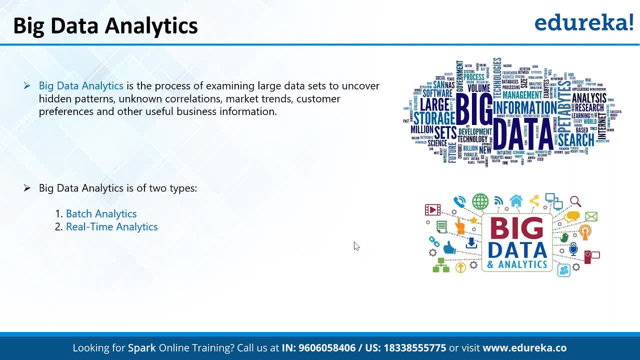 more accurate reports so that we can keep the customers happy. then, when it comes to banking and top finance domain, again, we do have fraud detection algorithms running. so whenever any abnormal transaction takes place, right, your banks or your credit card companies will be blocking the card, uh to to stop that fraud transaction. and what will happen eventually you'll feel happy, right. so 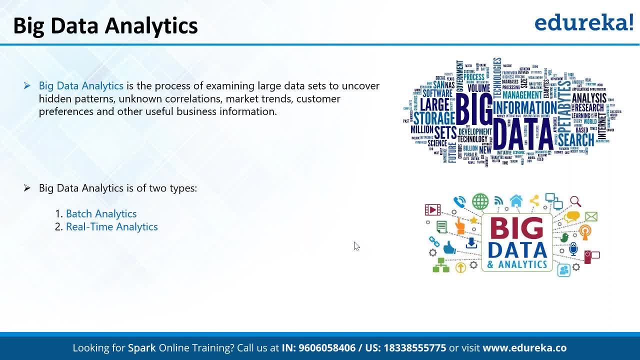 it's like in each and every domain, be it the energy- uh uh. energy domain beat the banking and finance social media uh b from. in each and every domain, we do have huge amount of data and we are interested in doing the analysis on that data. so big data analytics is is all about doing the 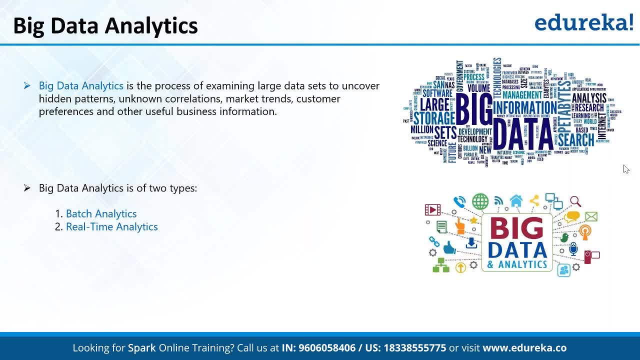 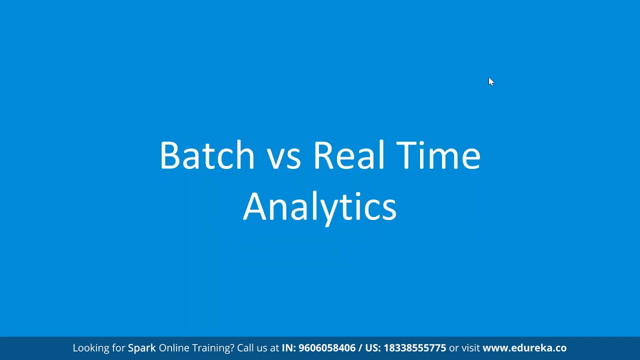 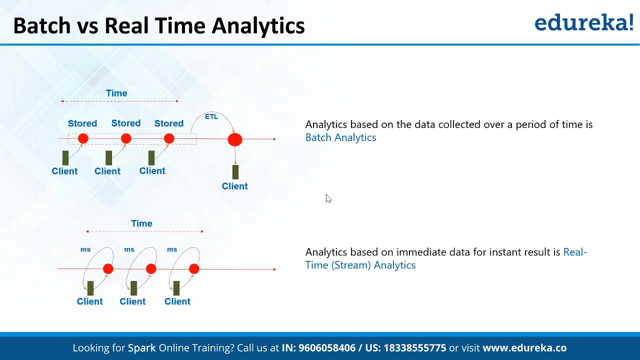 analysis on huge amount of data which has got varieties and also which is getting generated at a very high speed. okay, so now, when it comes to big data analytics, it is of two types. so we do have batch analysis and we do have real-time analysis. okay, so now, uh, let's talk about batch versus real-time analytics. okay, so, guys, when we talk about big data, 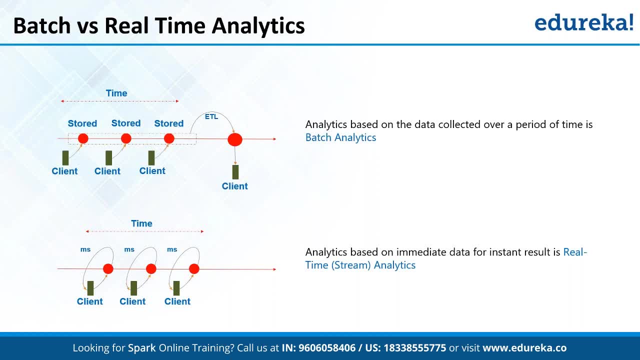 analytics? right, analysis on the data can be done in two ways, so one is the batch analysis. okay, so, batch analysis, what is it? as in every 15 minutes, you will be getting one file and at the end of the day, you need to generate a report on top of that data, right? so, as in what you see here, it's. 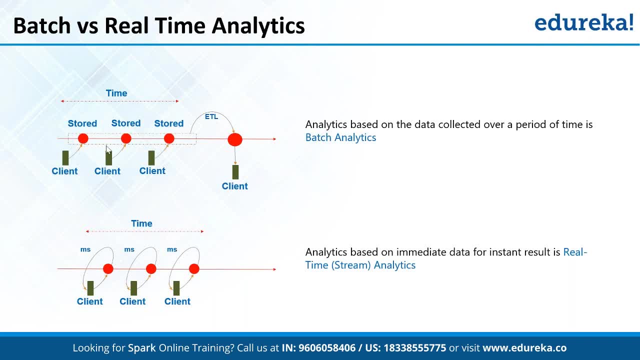 like client, is publishing the data data, right? you see, it is happening at regular interval and what we are doing at the end of the day, or as in at the schedule time, we are doing the analysis on that data, right? so this is nothing but batch analytics. okay, when it comes to the real-time analytics, as 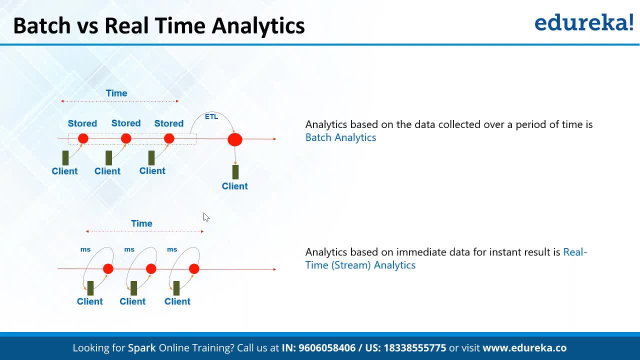 in as soon as we get the data from the client. purpose is to do the analysis on the data and to generate reports on that, as in i took example of i watch right, where we say that, yes, notification should be sent immediately to the doctor when the heartbeat is going low. what is that? that's nothing but the real-time analytics, right this? 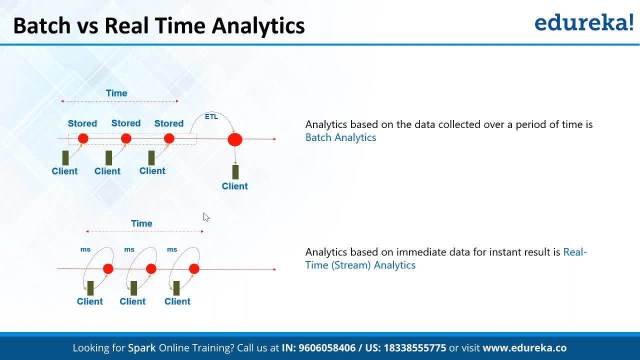 should not happen. that, you know, at the end of the day, report is getting generated and the end of the day, we are getting to know that, yes, something serious has happened because the heartbeat was low or all those things right. so that is the difference between batch and real-time analytics. 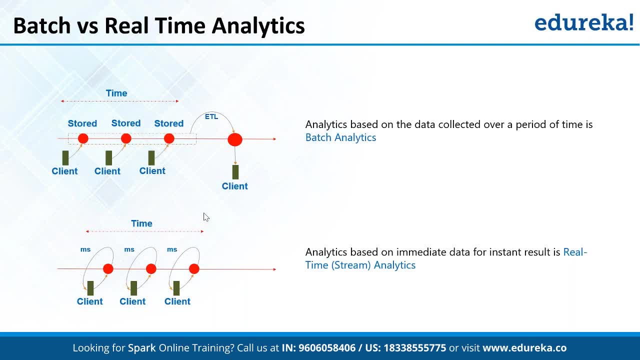 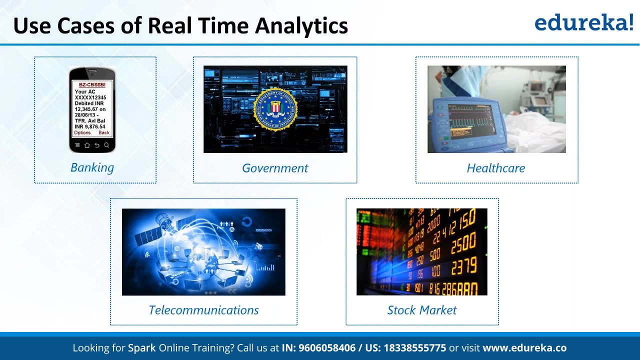 fine. so now for real-time analytics, we need a processing engine or we need a framework which has got high processing speed right. okay, when it comes to the batch data analytics, we do have hadoop, and when it comes to real-time analytics, we do have spark. so we'll talk about those. first of all, use. 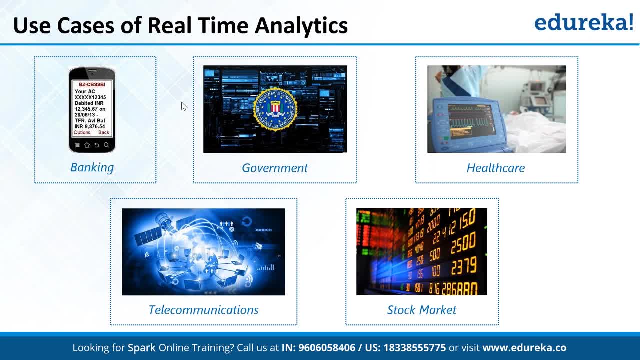 case of real-time analytics like banking: right, so you get message immediately on on your mobile phone that this, this, uh transaction has happened and this is the status right. health care: we are getting the reports immediately. stock market: we can see like what is the trend. telecommunications: right again real-time examples, then. government is is doing and is is having a number of use cases. 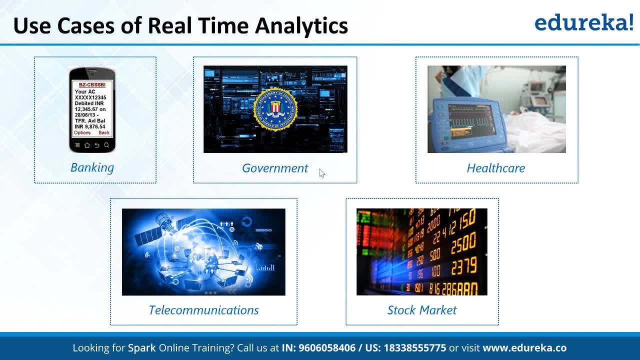 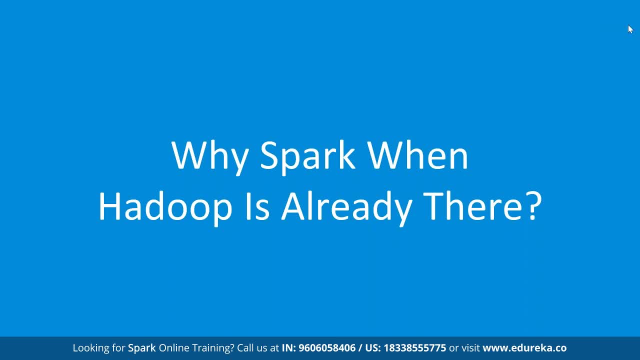 when it comes to real-time analytics, right. so now the point is: why spark when hadoop is already there? i'm not sure that how many of you are already comfortable with the hadoop, but i'll tell you so what we discussed here. we discussed that we do have two type of analytics, so we do have batch analytics and we do have real-time analytics. 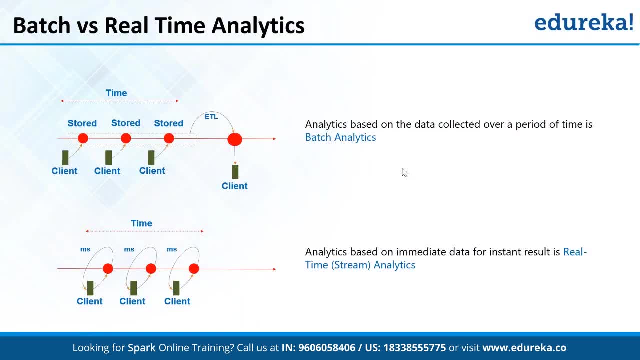 so when it comes to batch analytics, guys, so we use hadoop, okay. hadoop says that i will give the best result when the requirement is to do the analysis on batch data, but when it comes to the real-time analytics, we need high processing speed. so hadoop says: sorry, i cannot help you there, okay. 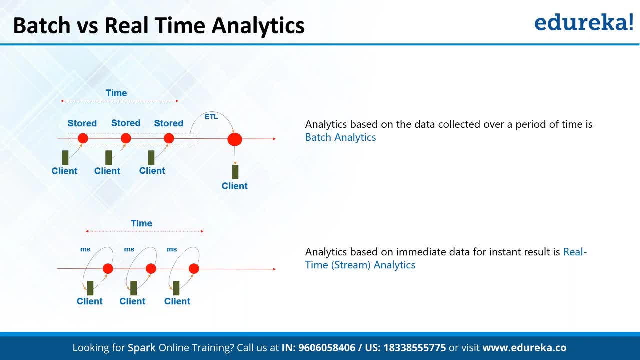 so i'll take one example here, similar. i'll ask him, and then we dumpling: the moment you open your facebook profile, what is the? what is a provide priority for facebook? to load the profile or to to show the updated uh news feed, or to show the friend suggestion? to show the? 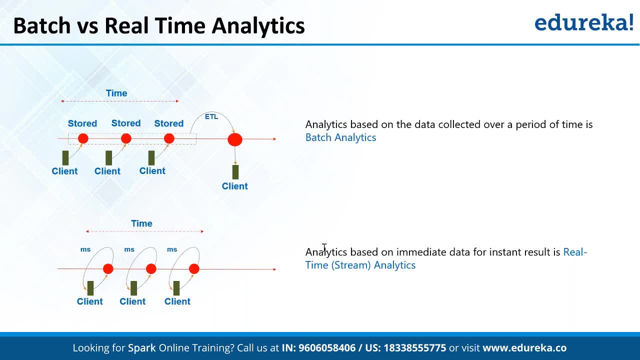 updated news feed, right, and then to, to, to show the friend suggestion. so these are two examples. so now showing the friend suggestions, it can be it. it is an example of batch analytics, fine. and showing the updated news feed is nothing but the example of real-time analytics, right. so these 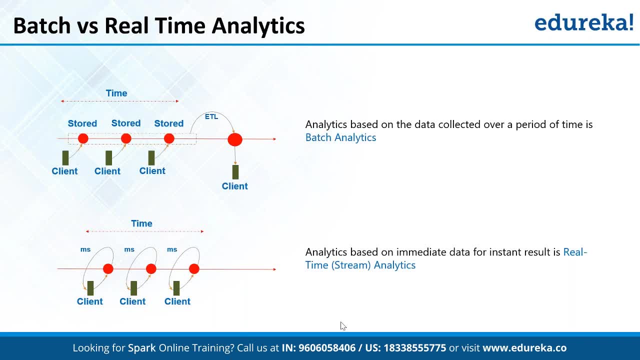 are the two different scenarios. and now for these two different type of analytics: right, facebook is using different, different tools or the components. so, for showing the friend suggestions, facebook is using hadoop- okay, and to show the updated news feed, facebook is using spark. right, and we will. 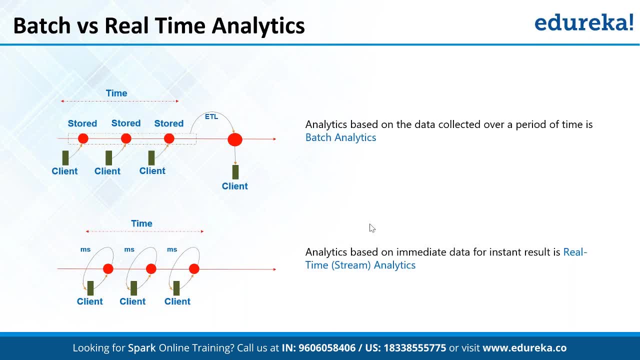 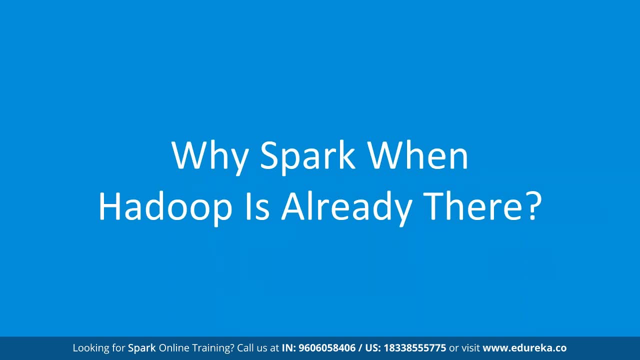 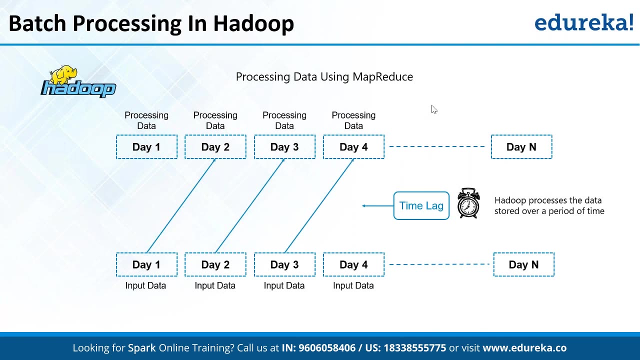 understand, like why facebook is not using spark for doing both the things. why spark when hadoop is already there, as in batch processing in hadoop- this is something which we have already discussed- as in hadoop is, you know, hadoop is suitable for doing the analysis on patch data, but not on the real-time data because there is some lag. okay, there is some. 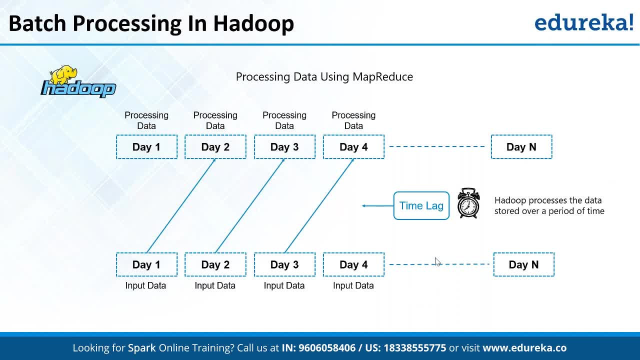 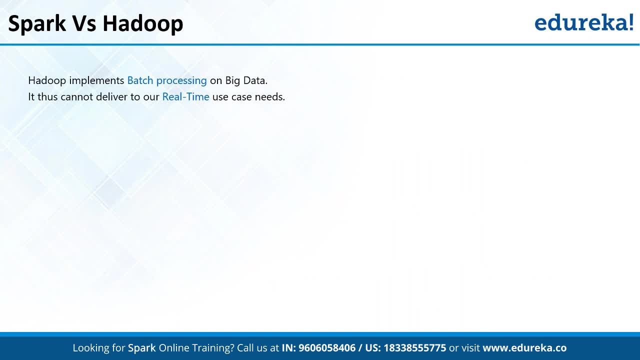 delay. but when it comes to spark right, spark says that, hey, there will not be any delay. you see, okay, so hadoop, it all works on batch processing, but when it comes to this spark right, it's like when it comes to real time. our data is like our requirement is to process. 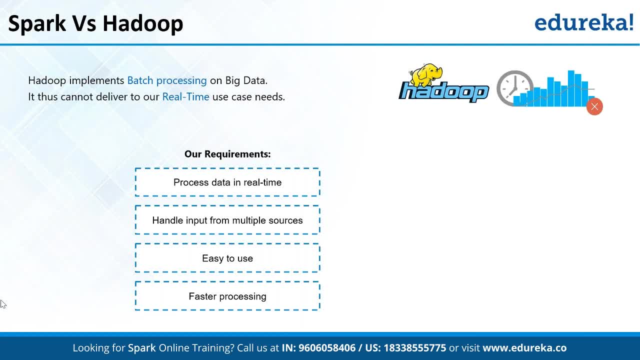 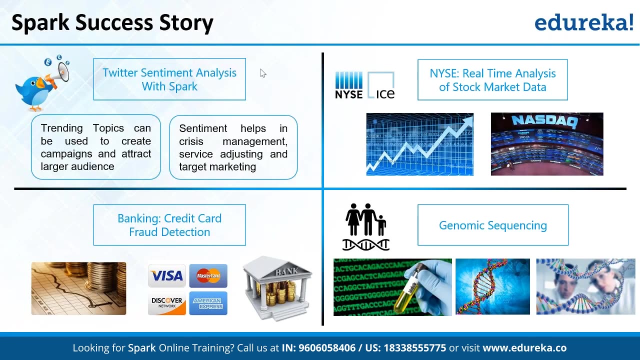 the data in real time, handle input from multiple sources, easy to use and faster processing. so what do we have here? it's like we do have spark, right, we do have spark. now. spark success story is like where and all spark is being used for twitter sentimental analysis. this question was asked like 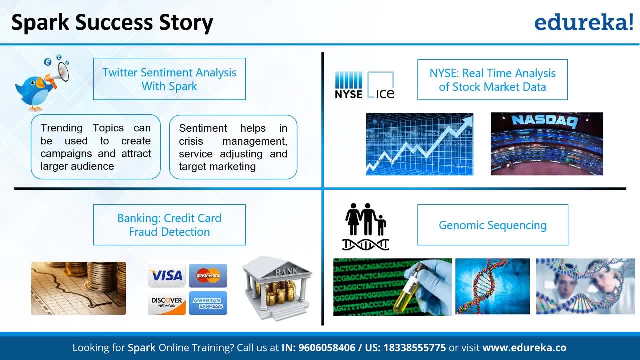 what do we do with the video data? as in: what is the sentimental analysis? as in: a company has launched a product in the market, okay, and they are interested in collecting the feedback, but they are not going with the traditional way where they are asking you to fill the form. so what? 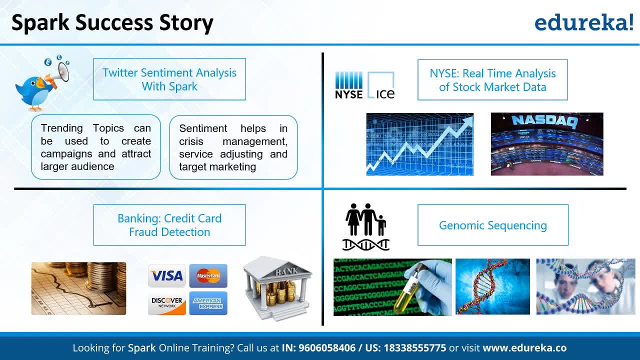 what they are doing there. they are going to the social media platform to see what people are sharing about that product. as in, you are extremely happy when you had purchased a new car. so what you did? you uploaded a video. i was kind of okay with that product, so i i tweeted something and there was someone else who uploaded an audio. so now, in order. 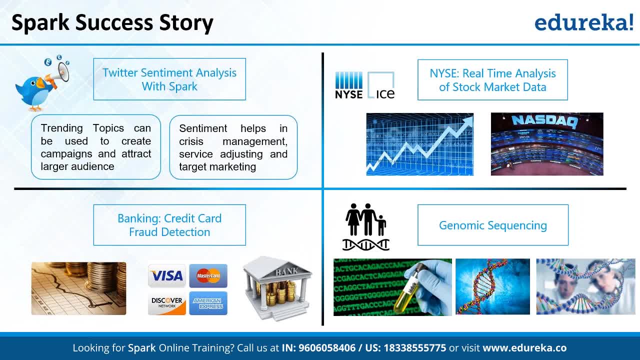 to get the collect feed in order to collect the correct feedback. right, there is a requirement to do the analysis on video data as well. right, so there is a requirement to do the analysis on video data as well. so we just cannot say that, okay, we are going to do the analysis on video data as well. 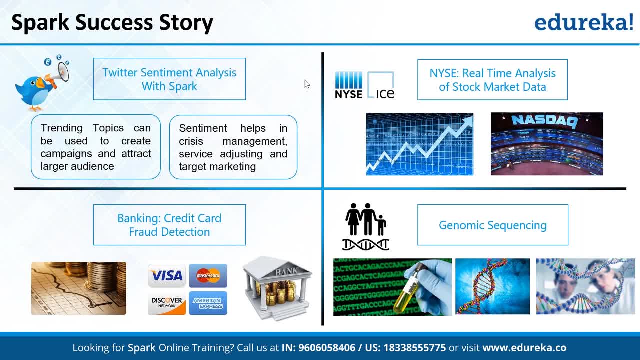 hey, we will be just uh, processing the text data to get the feedback right, so that is something which will not help, so we need to do the analysis on all kind of data, right, okay, so this is um right. so this is, this is nothing, but, uh, it's like sentimental analysis where 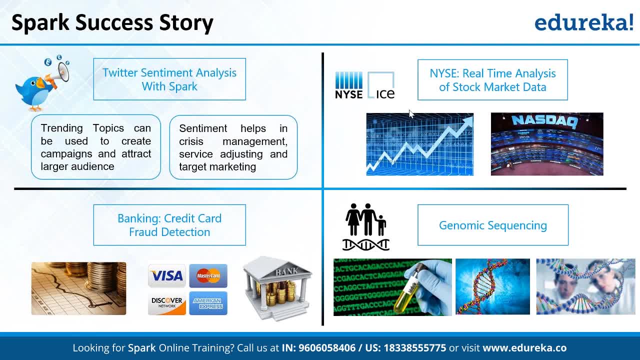 we are dealing with each and every kind of data. then what do we have? we do have new york stock exchange, where we do the real-time analysis on stock market data. right banking conversation, data and finance domain, then banking and finance domain. we do have example of fraud detection. 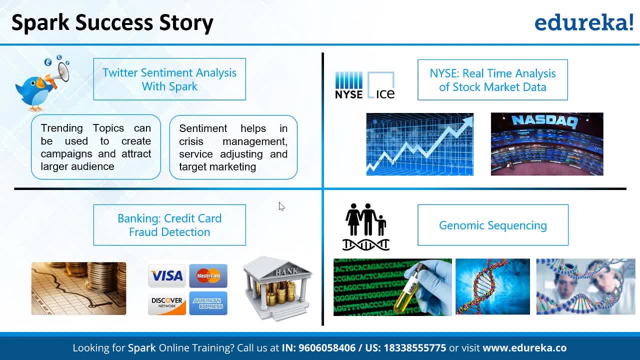 it's like whenever you make a abnormal uh transaction, your credit card will be uh blocked immediately. then we do have xenomic sequencing right. so now in in healthcare, right, there are n number of use case on big data analytics, as in uh there is. there is one startup called. 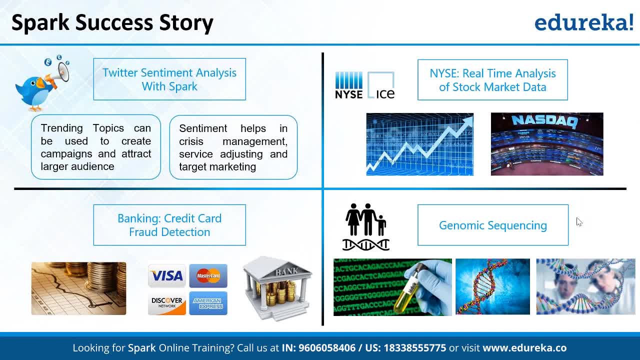 xenompatri. not sure how many of you are familiar with that or not. so what? what are they doing? it's like they will be collecting your blood sample and then they will tell you, like what are the diseases which you will have in future, so that you can, you can work, you can start working on life. 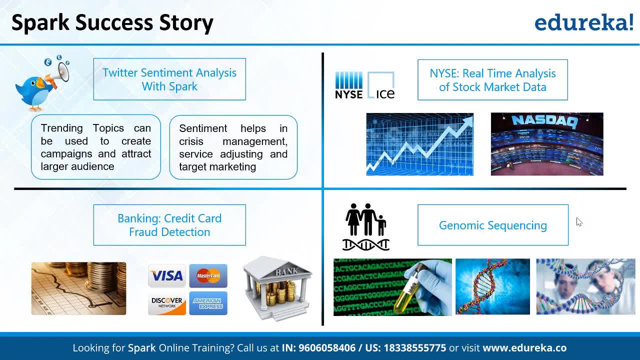 on your lifestyle from today onward. so what? how are they doing that? so they do have the patterns where they know that, okay, when this was a pattern, a person got this kind of disease right. so they do have that pattern. so they will be doing the analysis on your blood sample and then they will. 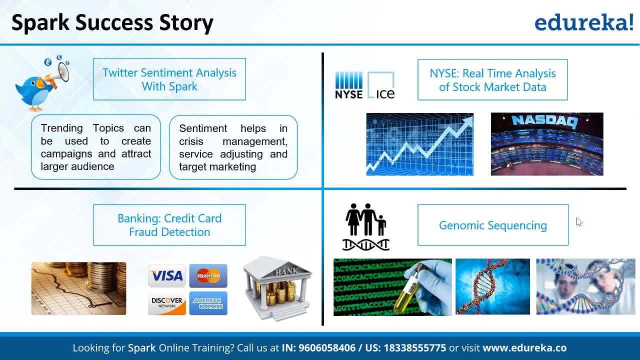 try to find the same pattern, and that's how they will be telling you that these are the diseases which, um, you can have in future. right, so these are the uh use cases. as in for real time analytics, uh, spark is being used everywhere, okay, okay, so now we will get the overview of spark. 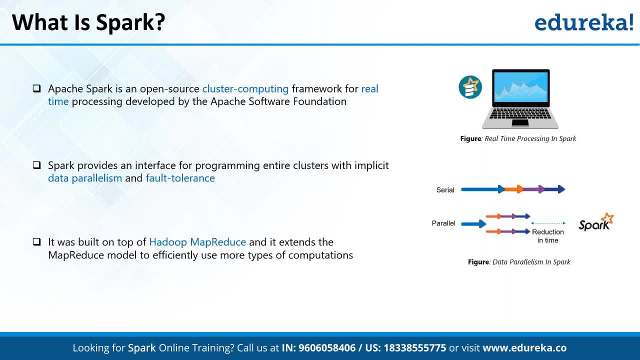 okay, so what is spark, guys? so, first of all, the main question which we have here is how spark is different from hadoop, as in when we say that hadoop is suitable for batch data and spark is suitable for real-time data, or what we say, we say that spark will give much better processing. 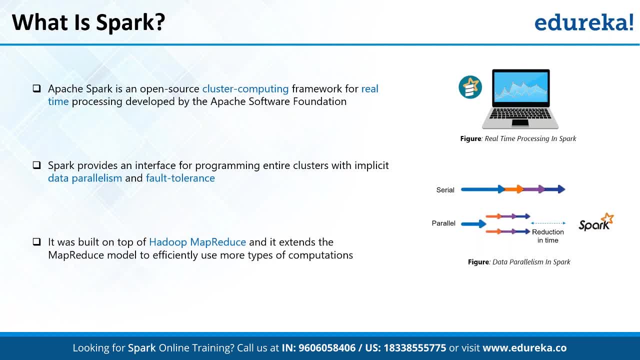 speed than hadoop. so what is the point here? or how the architecture is different, okay, so first of all, when it comes to spark, right, it's a distributed engine, as in. it will does the. it will does the parallel. it will do the parallel processing, as in. i do have, i'm a manager and i. 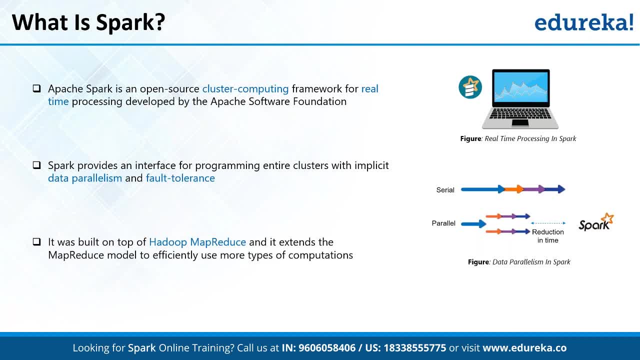 do have one resource under me. so point is whatever uh. point is whatever. i'm getting uh from a client, right? i'm asking only one resource to do that, so that resource will be taking some time to give me the result, right. but if i want to increase the processing speed, or let's say i've got 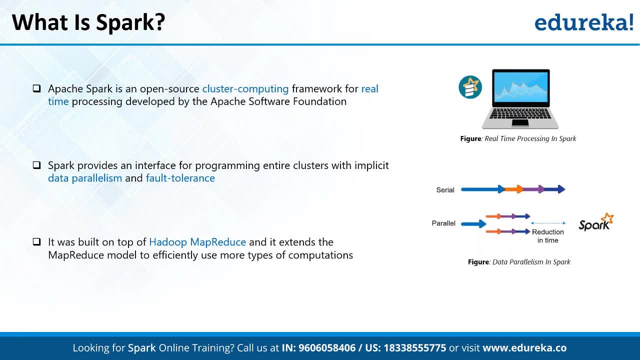 some critical requirement from the client and i'm like: no, no, we, we want the results quickly, quickly. so what i'll do? i'll pull up more resources and i will be asking those resources to work in parallel, right? so basically, that is nothing but a parallel processing. so spark works in the similar way. it. 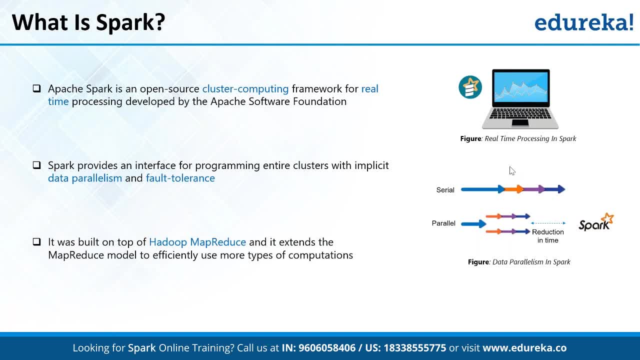 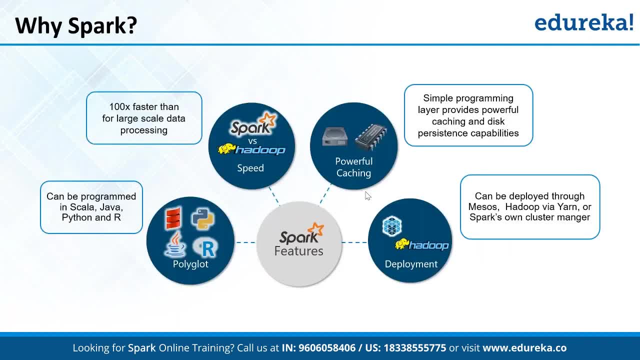 processing. okay, so what you see here, you see powerful caching as in it- is processing the data in memory. so now, if i ask you, like tell me what is expensive: disk or memory memory? right, yes, memory is expensive. so now, if we talk about hadoop and spark, right, hadoop is meant for doing the analysis on batch data, and what is it doing it? 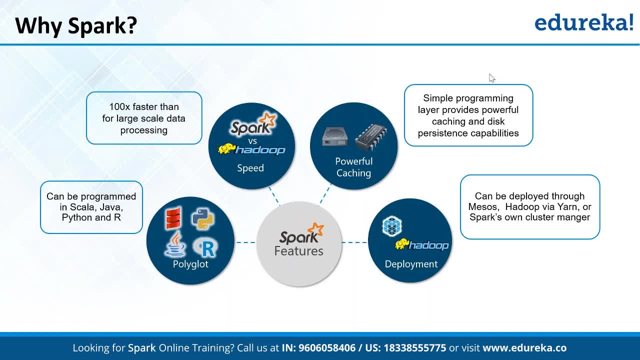 is doing the analysis on the disk. what it is doing? it is doing the analysis on the desk, right. so, basically, every time data is read and written to and from the test. but when it comes to spark right, what it is doing it is storing the data in the memory and then it is doing the 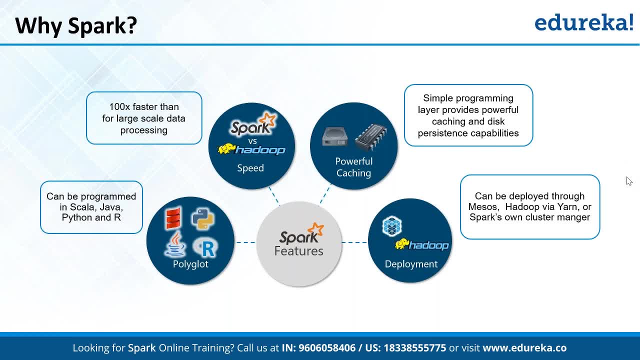 analysis on the data. so now, if we talk about this, right, if you have something in the cache, right, if you have something in the cache, then you know processing will happen faster, right? so this is something which is known to everyone. so, what spark does? spark says that i will not be. 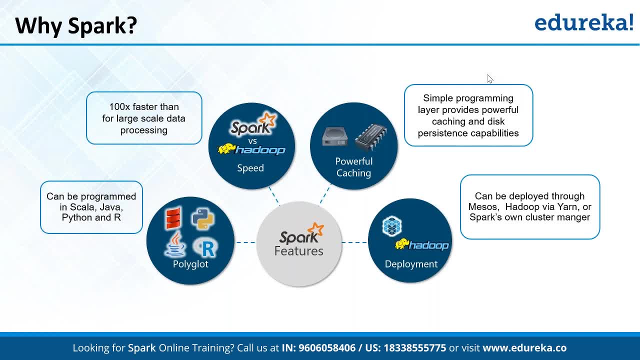 reading and writing the data each and every time to and from the disc. what it says? it says that i will be writing it to the memory and then i'll be doing the analysis, and that that's how spark is 100 times faster than hadoop. but the main point here is when it comes to spark, because it is doing- 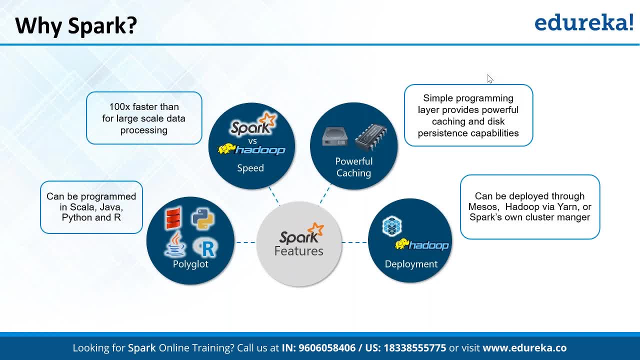 the analysis in the memory. it does not perform the analysis, it does not run the analysis. it does not work, but it does run. the is expensive, right, it is expensive. then hadoop because, in case of spark, right, we need more memory, okay. so now, uh, coming back to the same example of facebook. okay, because we know that. 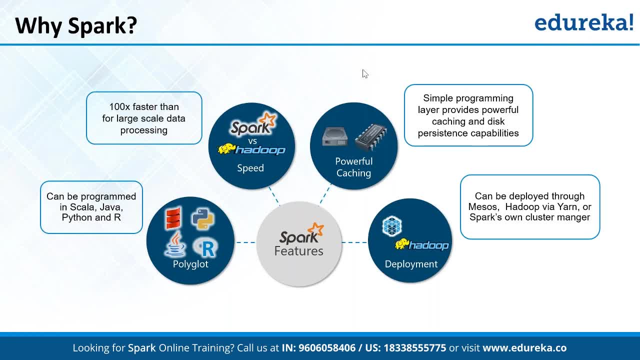 because we know that spark is expensive than hadoop. do you think that for showing the friend suggestions, facebook should be using spark? see friend suggestion is something like which we can show later as well, so do you think that facebook should- should be spending more amount on that? 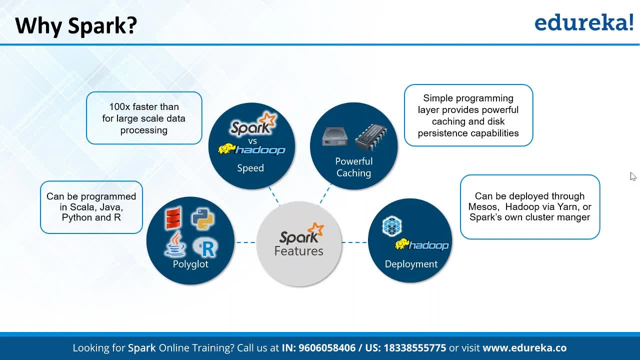 by using spark. no right, there is. there is no need. that's what right? so it's like that. it's like it's not that that spark has overcome hadoop or things like that. the only thing is based on your need. you will be choosing. uh, when i was, i was, it's like i had changed. 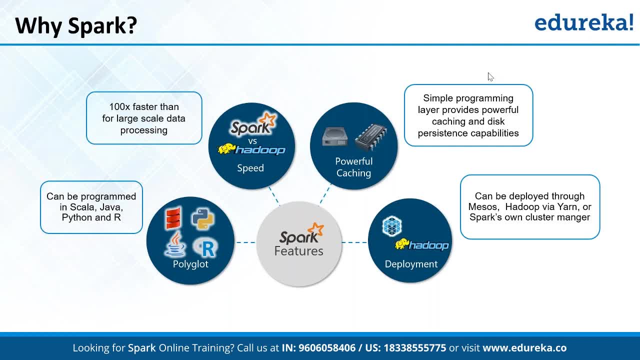 when i changed the organization- before changing right- i was working on spark, but when i changed the organization i was asked to work on hadoop right. so now normally people say that you know, spark is advanced version, so we should be working on that. that's in high demand. 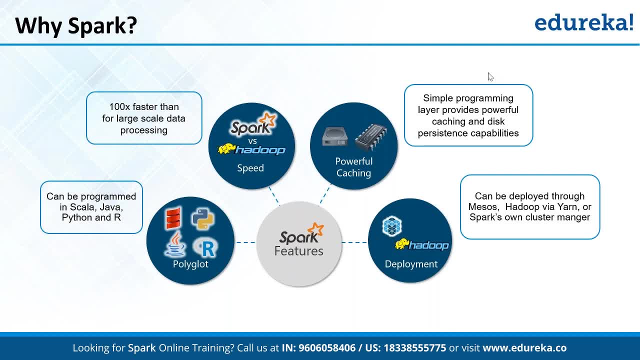 why are you working on hadoop? so point was that use case was difference different? okay, they clearly told me that this is a use case. that's why we are working on hadoop and that's why you will have to work on map reduce or hive or other things. point is it will always depend on the use case it will. 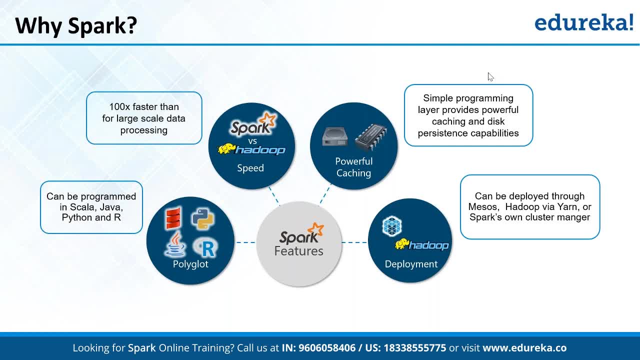 depend on the use case. so you should not be- you know, uh, you should not- be surprised if someone is asking you to work on hadoop today. okay, uh, for facebook messenger, right. facebook is using hbase for showing the timeline events. facebook is using cassandra, facebook is using mongodb as well, so the 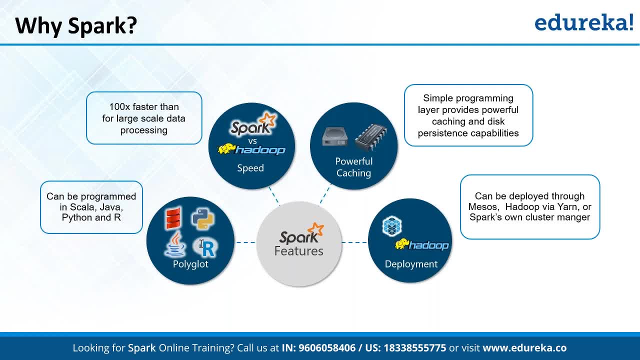 point is based on your need or based on your use case, you will be choosing the ecosystem component. so now when you go for interviews, right, they will be asking you: like, on what component did you work, right? so expectation is not that that if i have worked on spark, even you would have worked on. 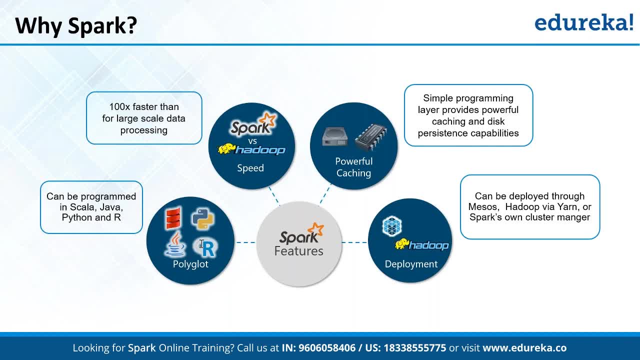 spark for sure, right? no, because for your project, use case might differ. so that's why you were working on different ecosystem components or tools, right? so that's why, whenever you look at the job description for a big data profession, right, it will always differ. someone would have mentioned: 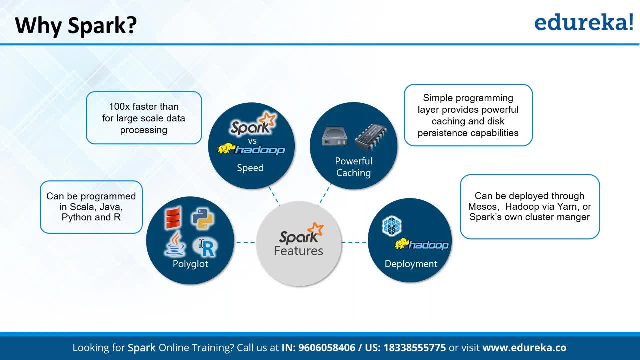 mongodb and cassandra. someone would have mentioned spark and kafka, but the point is, if you are interested in pursuing your career in big data domain, you need to be flexible, you need to be adaptable and you need to have very good learning skills, because things are changing pretty much fast. so you cannot say that, hey, i worked on hadoop and i'll work only. 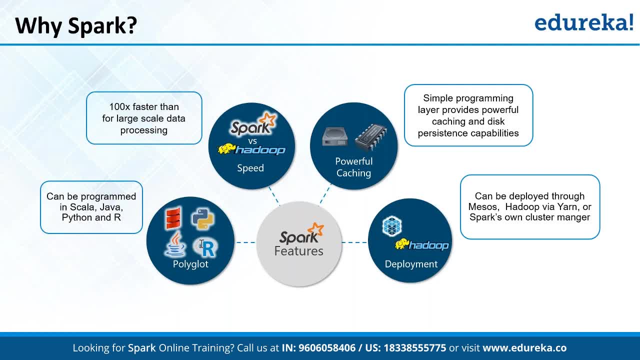 on that. no, you, that's. that's something which is not happening today, so that's why you always you need to keep yourself updated. so now, um, that was about in memory processing. right, because it is doing the processing in the memory. that's why spark is 100 times faster, okay, so yeah, now when 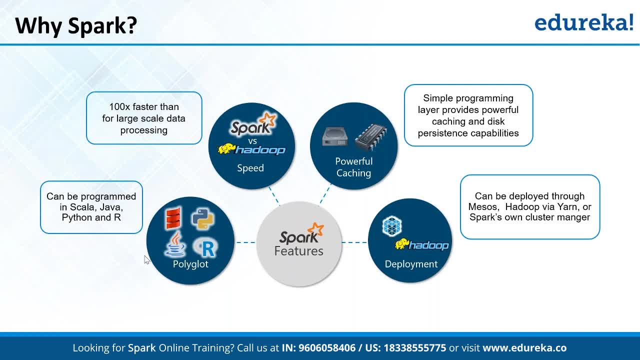 the implementation of business logic. when it comes to spark, you can use scala, java, python and r. you can use any language. so basically, python and r are being used for statistical analysis. mostly. okay, when you uh there is a need to do the analysis, uh, whenever there is a need to do the. 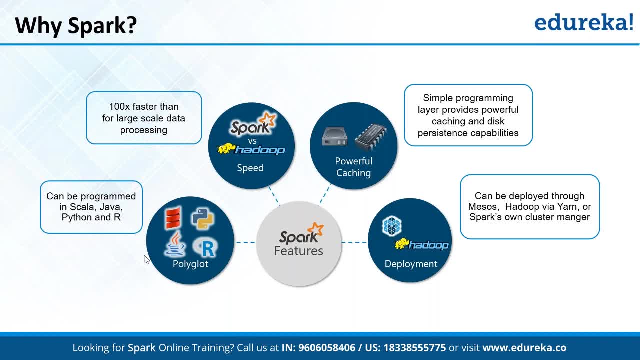 statistical analysis. we will be using python and r, otherwise scala and java, but java is not being used much these days. it's always about scala and python. fine, so now when it comes to the deployment. so basically, we do have a framework for uh managing, so as in like, it can be deployed. 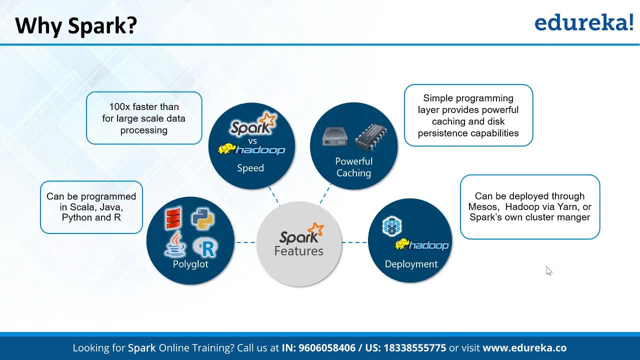 through mesos, hadoop, yarn or sparks, own cluster management. so not sure like how many of you are comfortable with yarn or how many of you have uh, how many of you have uh worked on uh, basically hadoop right. so it's like the point is, as uh deployment can be done in n number of ways, 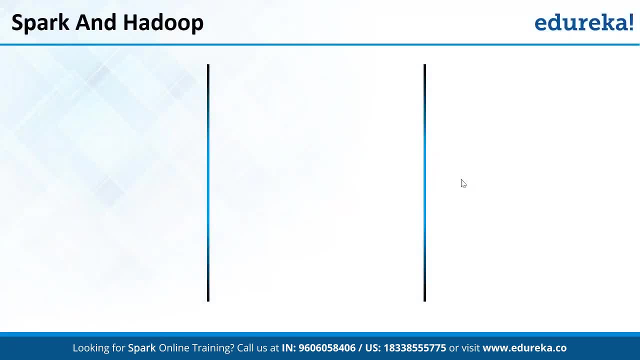 okay, using hadoop through spark. so now uh point is how spark and hadoop are interrelated. let's understand, okay. so basically, spark will be running on top of our distributed file systems. the point is, first of all, we need to store the data in distributed manner, as in when a manager wants. 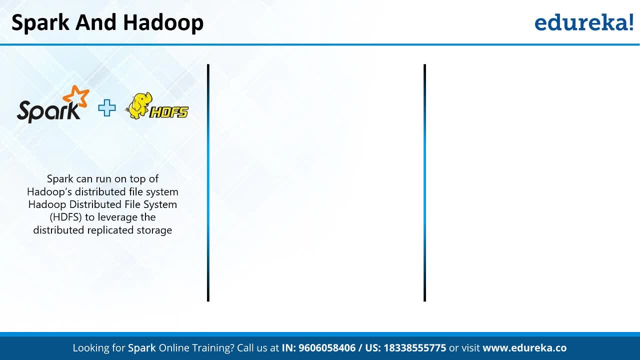 its resources to do the work in parallel. so what is the first job of manager? first job of manager is to do the distribution of the work. so that's like giving the data to the resources so that resources can do the analysis on that. so when it comes to spark, right spark would be running. 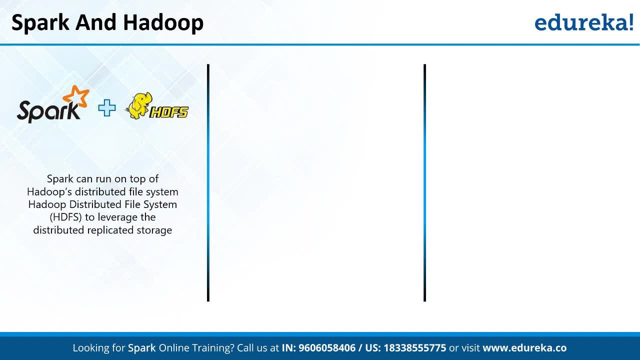 on top of a file system. it can run off hdfs, and hdfs stands for hadoop, distributed file system. so now map reduce. basically again, it's nothing, but it's a processing engine of hadoop. so it's like even this processing engine can be used along with spark, but usually we don't do that. 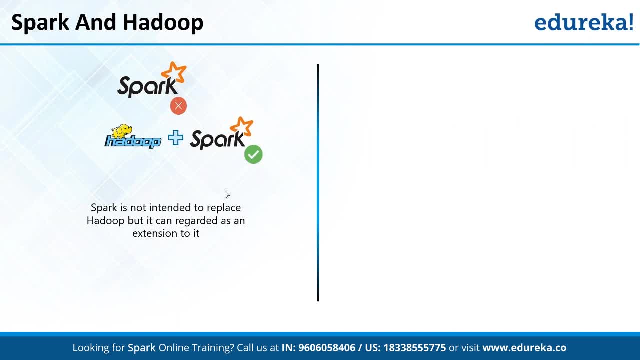 okay, spark and hadoop. so basically, spark is not intended to replace the hadoop distribution. so it's not intended to replace hadoop, but it can be regarded as an extension to it. right, based on your use case, right, you will be choosing. like i told you that facebook is using both, like spark. 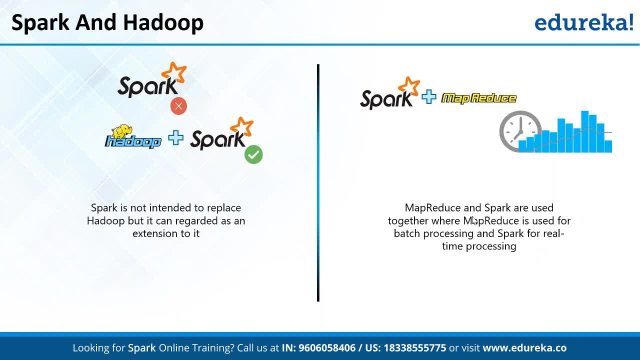 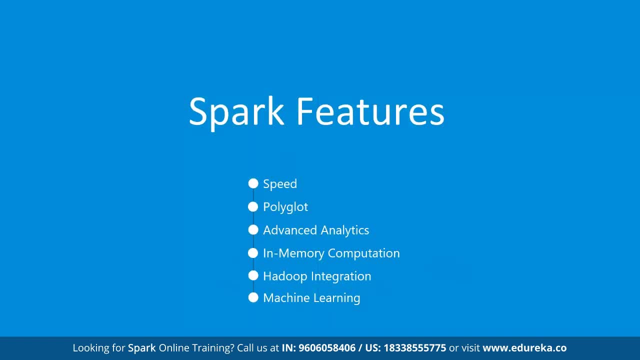 and map reduce. map reduce and spark are used together, where map reduce is used for batch processing and spark for real-time processing. okay, so now what are the spark features? as in speed, it is 100 times faster than hadoop. it is polyglot. as in different, different programming languages. 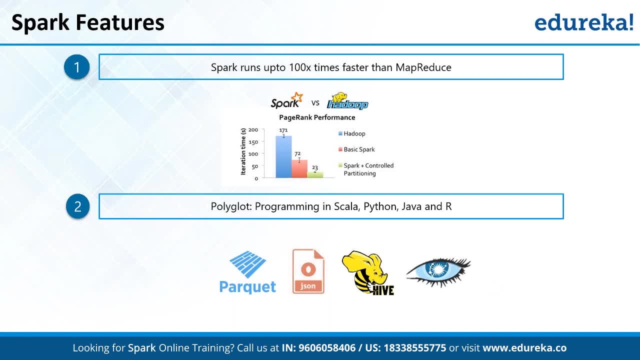 can be used, as in: you can implement the business logic using skype, or you can implement the business logic using java and r, and also it can work with different different uh types of file formats, as in json parquet file format. and then we do have high, so using high you can write sql like queries. 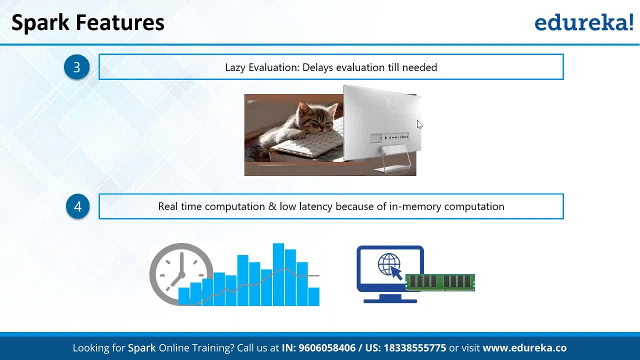 okay and also, when it comes to spark it, it does the lazy evaluation, so lazy evolution, as in um. first it will be taking your instructions and whenever you ask it to show the result, then only it will be executing the set of instructions. okay, and real-time computation and low latency because of in-memory computation. it's like 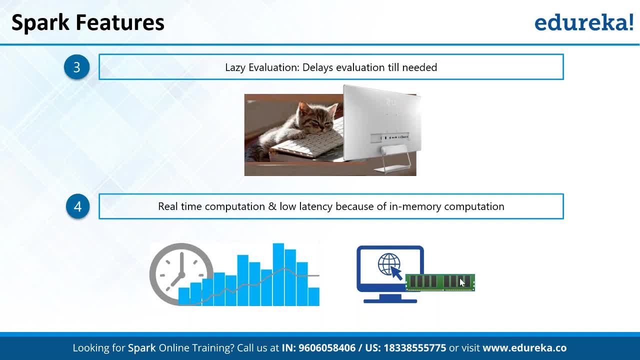 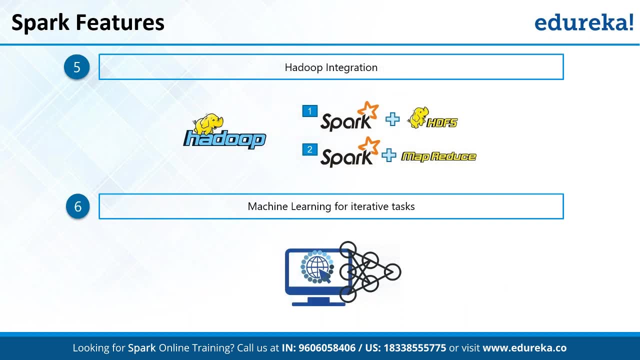 what it will be doing. it will be processing the data in memory and that's why it will be taking less time. okay, hadoop integration- integration of spark can be done easily with hadoop and also machine learning for iterative. yeah, so it's like spark was mainly designed for implementing the 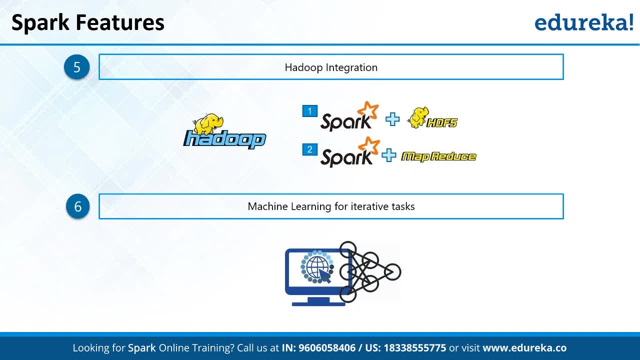 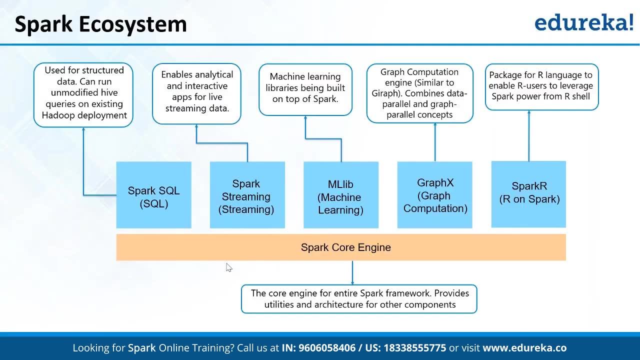 machine learning algorithms where we say that analysis on the data will happen again and again and that's why it is always suitable for keeping it in the memory. okay, so let's uh move on. okay, now spark: ecosystem components. so, guys, this is what are the capabilities of spark. so now i have 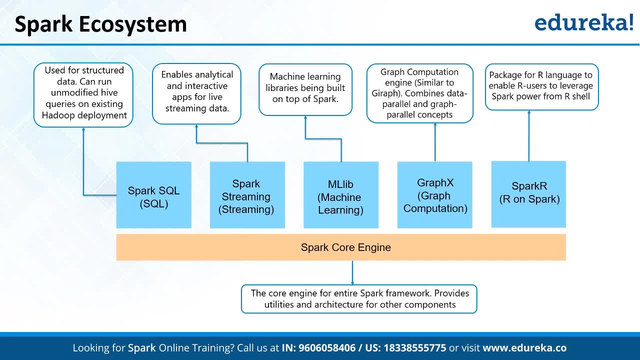 a question here like: why spark, when? very, very simple answer to this question: first of all, because spark has got n number of features. and then, when it comes to the spark ecosystem, just one installation of spark and you can do n number of. It's like you can implement n number of use cases. 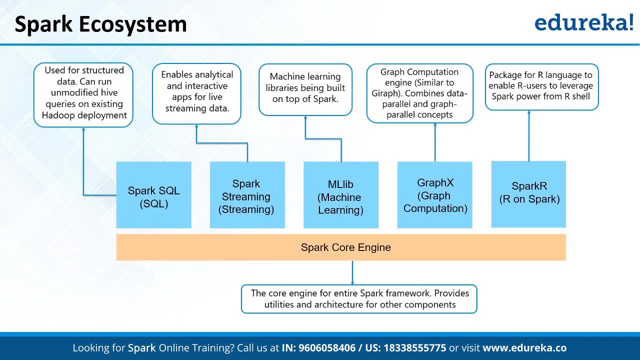 as in: if you have installed spark right and if you have need that, if you have need to do the analysis on structure to data right, or it's like if you want to write the sequel like queries to do the analysis on that data, We do have a module called spark sequel right. 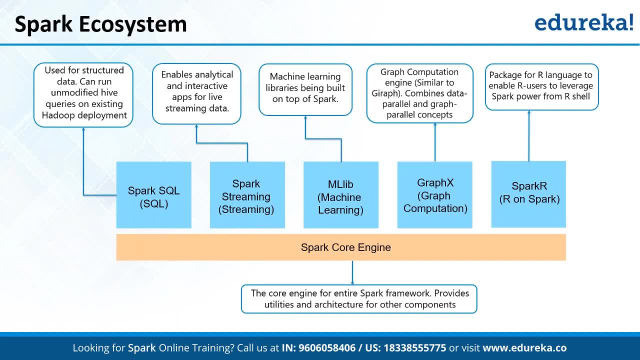 So now, if you have the need to do the analysis on real-time data, which is nothing but spark streaming, We do have a module for that. So when we when we talk about spark streaming, right? So basically, it is a module in which we have got n number. 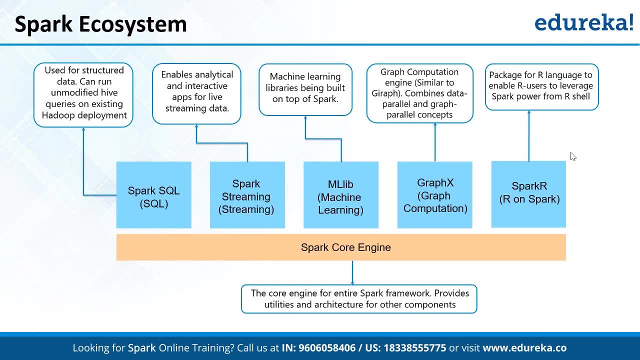 of inbuilt functions and with the help of these inbuilt functions. right, You can do the analysis on real-time data easily. Now, if you have need to implement the machine learning algorithms, what you can do is, again, We have the module if you have need. 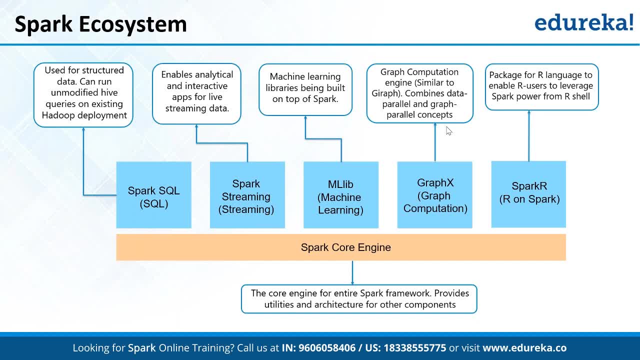 to do the analysis on graph data, again, you can use spark and then spark are. or if you want to write our queries, you can use this. So now let's say that spark is not there, or let's say that you know you don't have spark, or you are not using spark. 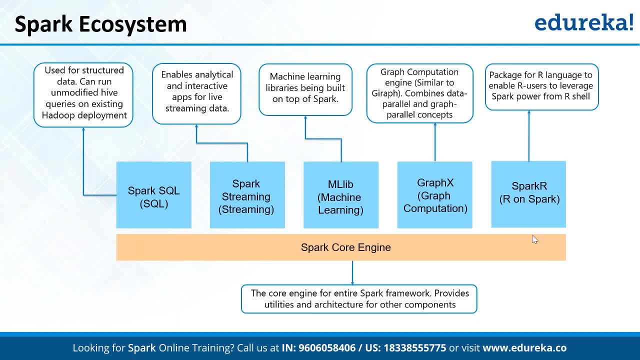 If spark is not there, you will have to install different different components. as in for doing the analysis on graph data, you will have to install different component which is neo4j or graphics. then for machine learning you will use my heart or any other tool then for spark streaming. 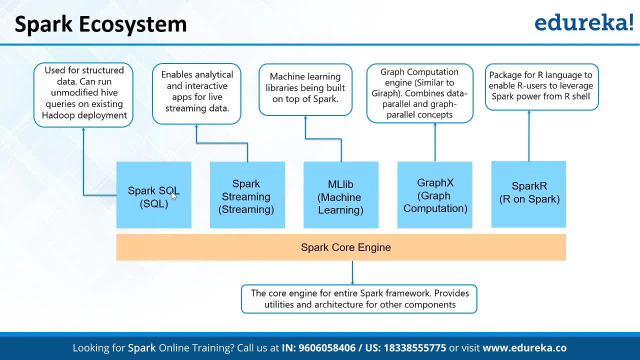 You can use a storm then for writing the sequel, like queries, you can use hive or something else. So the point is it's it's very easy to use just one installation and you're done. you don't need to make any change in the cluster, and whenever your requirements. 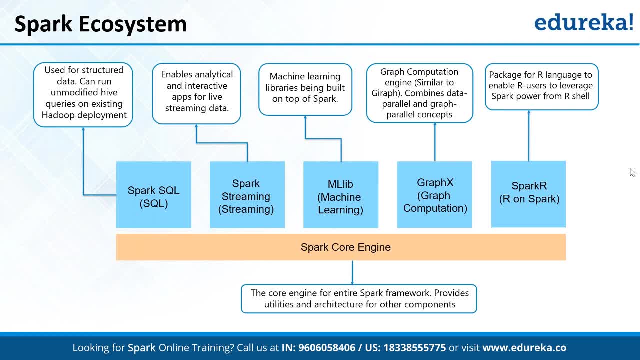 in this, you can easily take the advantage of these components. Okay, so this is this is why a spark is being famous again. when you go for the interviews and if you say that you know you're working on spark, they will ask you for sure. 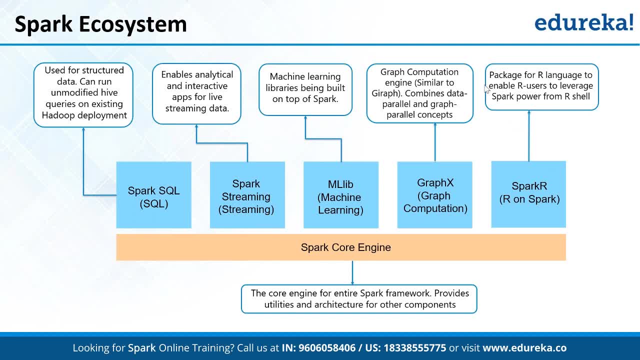 So which module of spark did you use? you need to tell them if you used on, if you worked on spark streaming, or if you used on Spark mlb or spark sequel. right, If you are working on spark does not mean that you have got expertise on all these. no, not at all. fine. 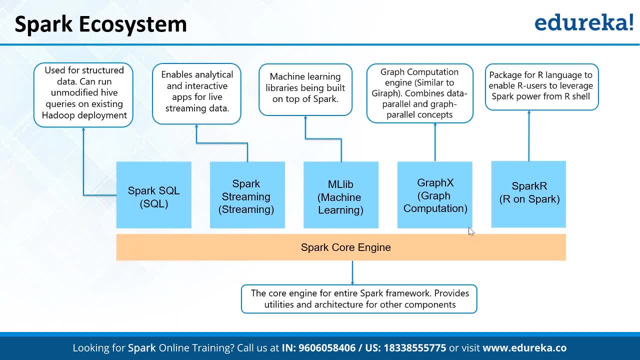 Again, it will depend on the requirement and that's why you know some organizations are just using mlb feature of spark, Some are just using graphics, Some are using spark streaming, So it will always differ. Okay, Let's move on. 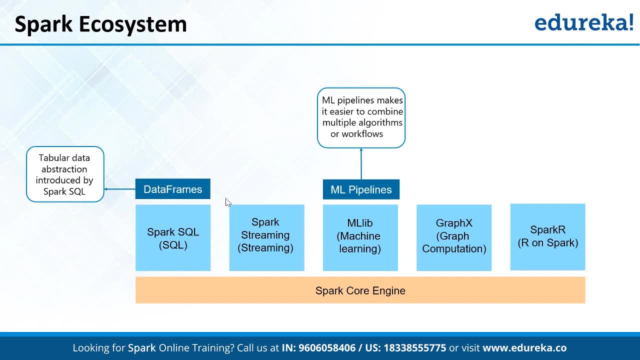 So yeah, basically spark. Like I told you that, using this module, you can write sequel like languages. as an, you can store your data in form of rows and columns so that you can write the sequel like queries. Right then, we do have spark mlb using. 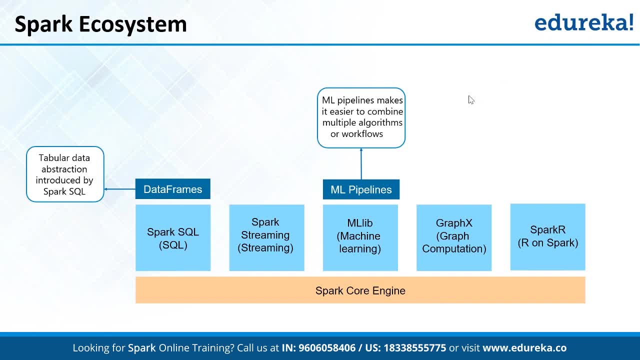 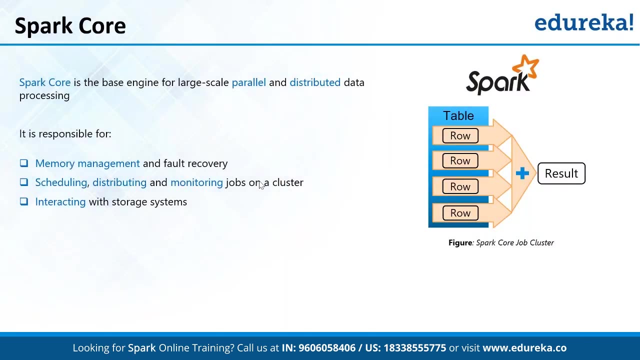 which you can implement the machine learning algorithm. when it comes to uber, right, uber is using spark mlb for doing the analysis on the data. Okay, let's move on Spark core. as in it's, it's the main processing engine. So, as part of this, like whenever we do the detailed discussion, 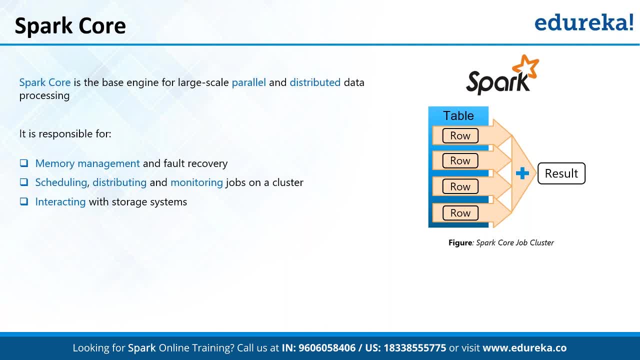 of Spark or right, so we will understand, like how it does the memory management or fault recovery. So what I said? I said that, yes, when we discuss architecture, then we will be discussing all these things in detail. So this is the same thing here: memory management. 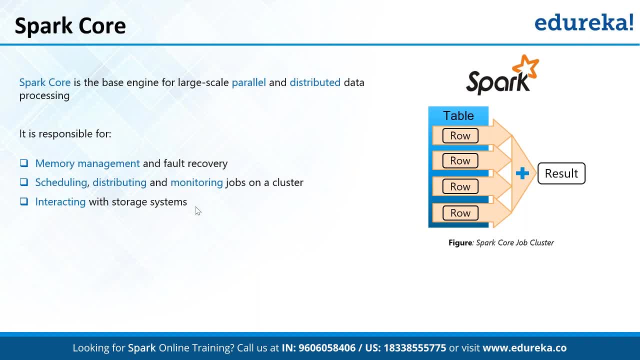 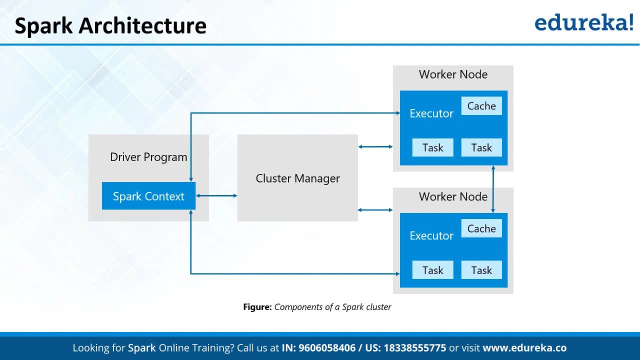 and fault recovery, scheduling, distribution and monitoring jobs on the cluster interacting with This system. so you will understand. so, when it comes to the spark architecture, guys, we do have a master slave architecture as in like. we do have as in like. what we have got is we have caught up. 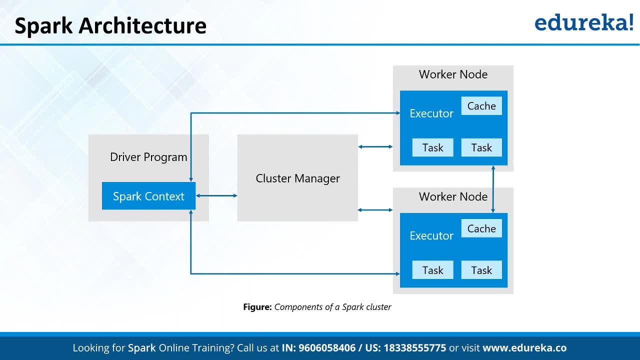 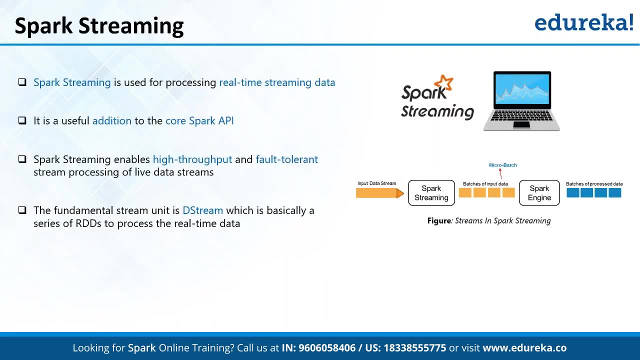 We do have master, or the manager, which will be giving the instructions and then, accordingly, workers will be working on the assigned task. Okay, So what is spark streaming? spark streaming is nothing but doing the analysis on the real-time data. So now the point is when you are getting 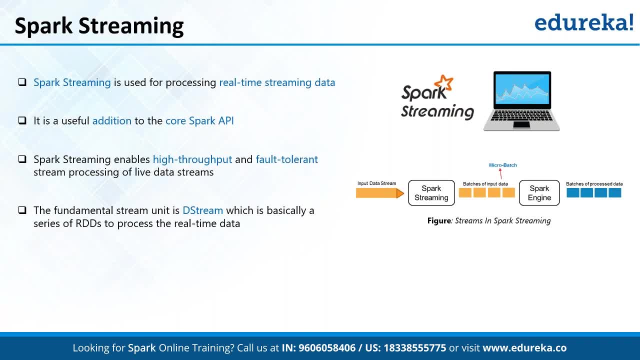 the data continuously. how would you be doing the analysis on that? So for that, we do have spark streaming. So spark streaming is nothing, but it's a you know, it's a modular feature using which you can do the analysis or real-time data. 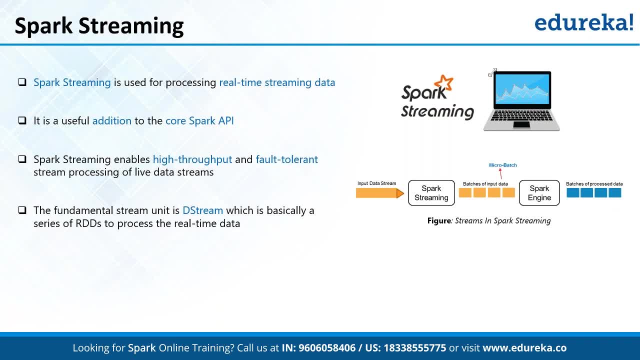 So how it works. So, basically, so how it works, It's like it will be creating the batches of the incoming data, but it's like, when it comes to the batch creation, this batch can be of millisecond or microsecond, right, So batches will get created. 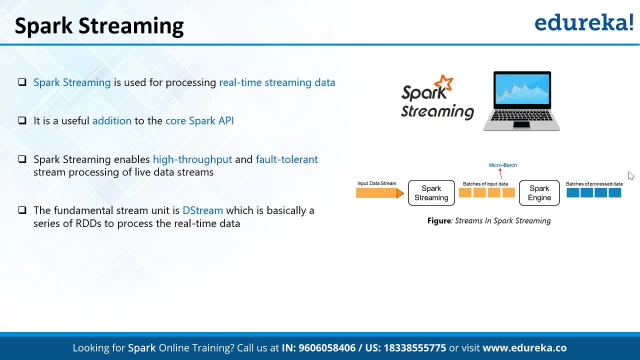 and then it's the code spark Only okay, Top. and says Hadoop also have yes, Yes, top. and so the point is, if you have got understanding on Hadoop already, it is very, very easy to do the analysis, or it's very easy for you to work on spark. 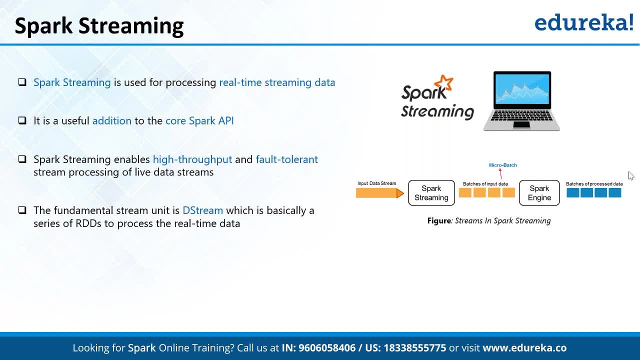 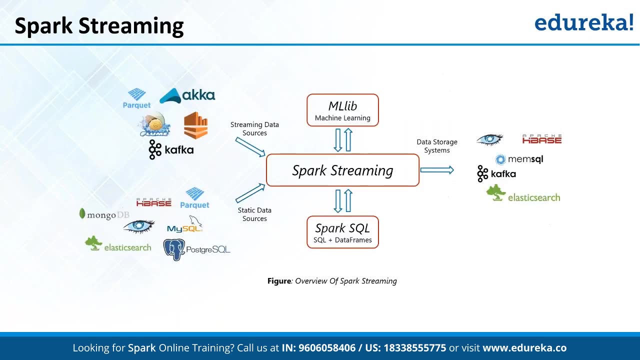 It shows one stream. can it handle multiple streams? Yes, it can. It can handle multiple streams as well. Okay, Okay, So now, when it comes to spark streaming, like this question was asked, like how the streaming data is fed to spark, right, 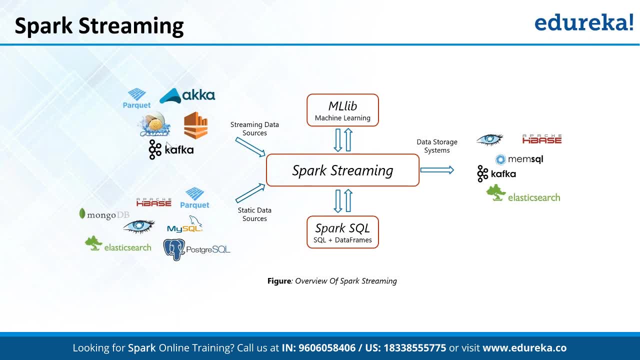 So what is that? I said that we do have Kafka, but along with Kafka we do have other tools, like we do have a car, We do have flume, So streaming data sources. So these data, will these tools right? They will be feeding the real-time data to the spark and 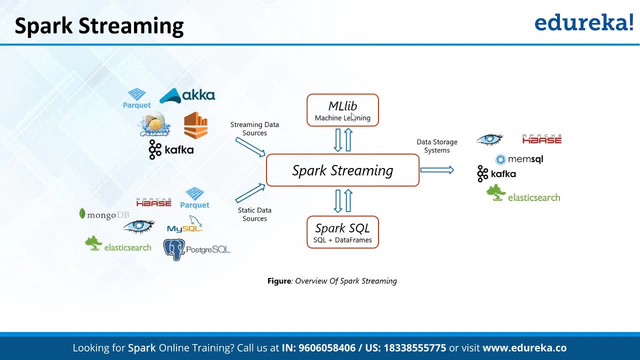 then on the real-time data, It's like we can run or we can implement the machine learning algorithm, So what we can write the sequel like query Is to do the analysis on the data. Okay, so spark streaming. So basically, what you see here is, let's say that there is. 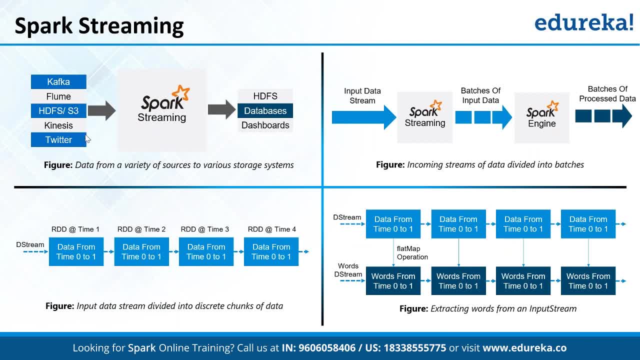 Kafka. right, Kafka will be getting the data, Let's say, from Twitter, continuously. It will be getting, it will be feeding it to spark streaming. and what will happen? like? either it can go stored to HDFS, which is nothing but a storage system. That's why I said that first of all. 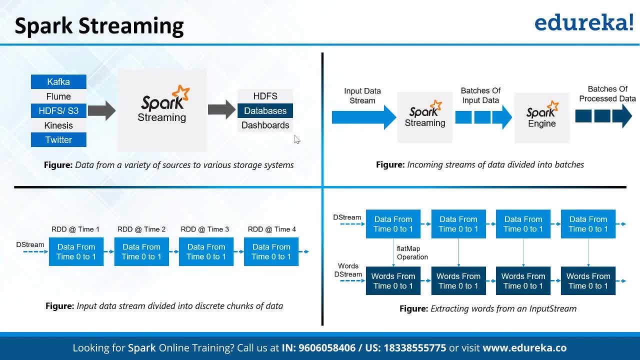 First of all, what we need to do is: it's like we need to store the data. So, when it comes to the data storage, right, you can, you can. you can store it in HDFS, or you can store it in database or in a dashboard. 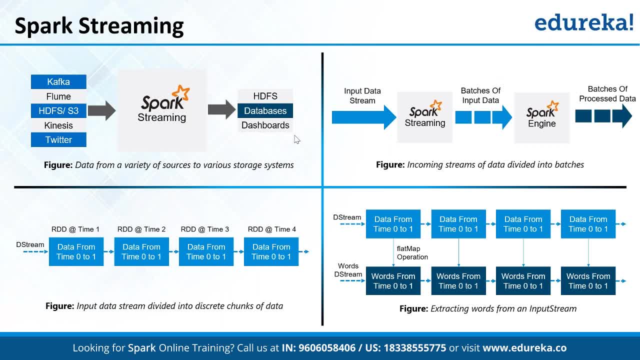 right. So now, once we have this streaming data, what will happen? So it's like input data stream right, batches will get created and then it will be fed to the same code: spark engine. So it's like batches will get created as an. it says that this: 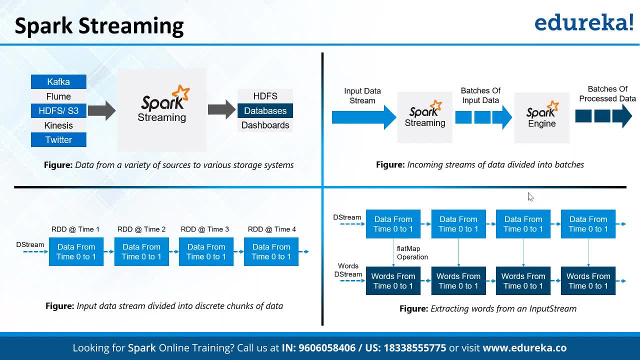 is the badge from 0 to 1 second, 1 to 2 second and that's how data would be flowing. So it's like if you have got understanding, of course, park, it's a very, very easy for you to work on the Spark streaming. 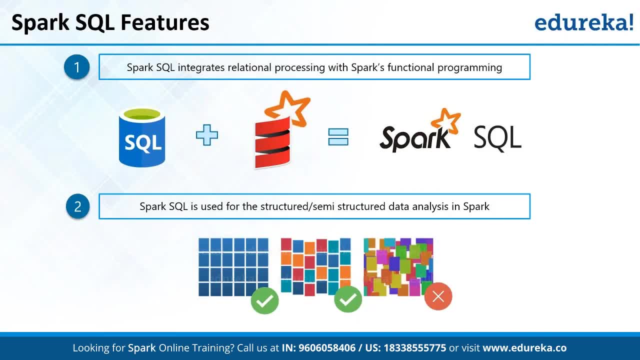 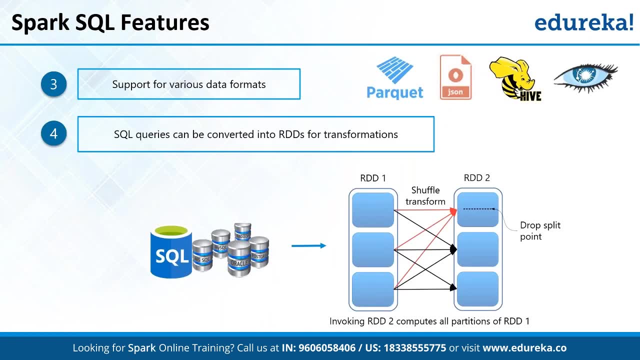 Okay so a spark sequel feature, as in if you already know, like, how do you write the sequel queries. It's very easy to work on Spark And it supports different, different file formats. Okay so, as in the spark sequel, it will be making your job easy. 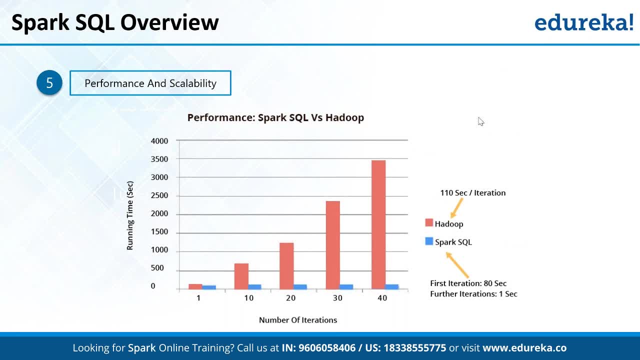 Okay. so it's like, if you do, if you come from a sequel background up, your job is very easy. You just need to write the sequel query, You just need to get the understanding of spark framework and then you can write the sequel query. 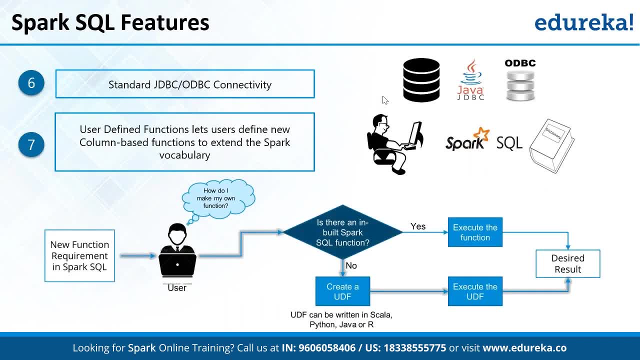 Okay, then we do have spark sequel features. Yeah, JDBC ODBC connectivity. So when it comes to Kafka, right, Kafka is not limited to the integration with spark. Kafka is capable of placing the data to different, different databases as well, So it's like you just need to have a connectivity to that database. 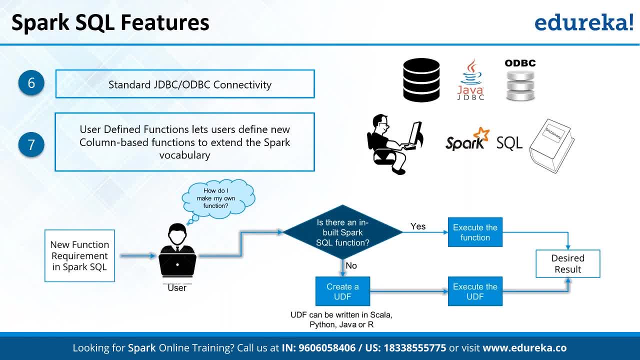 And like those who are working on Java right, or those who are dealing with real-time, with those who are using code Java right. So our advanced, even they are using Kafka. So it's not that that it is limited to spark. So, when it comes to spark, sequel. 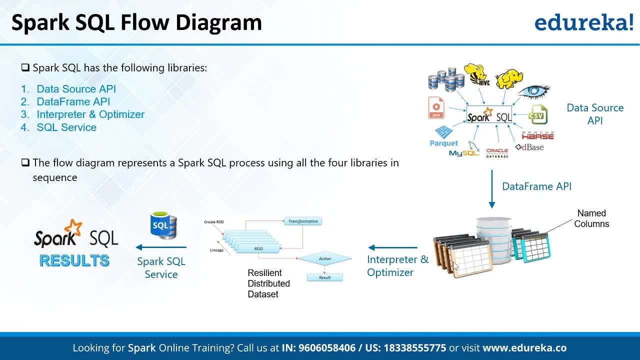 right. you will be getting the data from different sources and then data frames will get created and you will be writing the sequel query and internally it will be running the sequel query on top of the core engine. as in now, you don't need to write a complex. 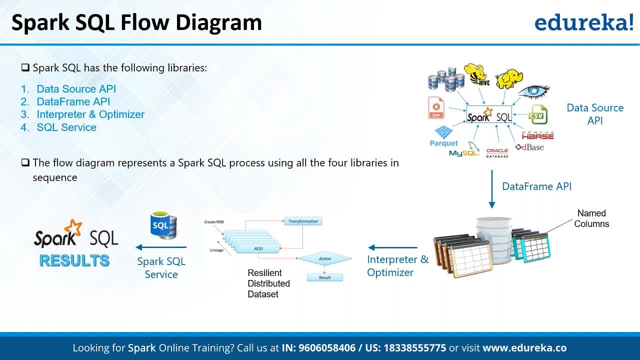 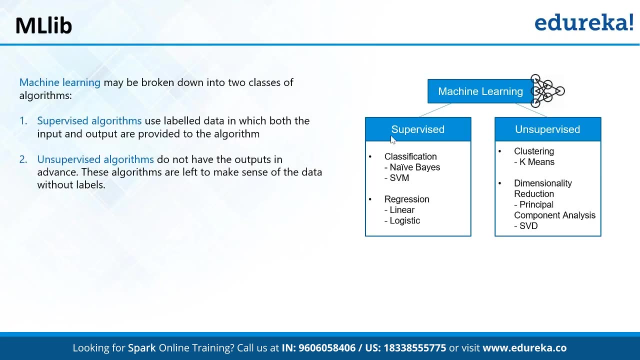 Program, Let's say in Java, and scale or invite, and it says that: hey, I work as an interpreter, You just give the sequel query to me, I will convert it so that it can be understood internally by the processing engine. Okay, Now, when it comes to the ML labor, when it comes to the machine, 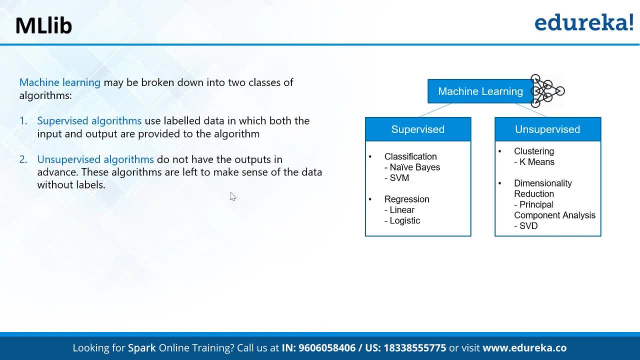 learning right. So spark has got modules using which we can implement the machine learning algorithm. So when it comes to machine learning algorithm, we do have, we do have a, we do have two types. So for algorithms is like we do have supervised and unsupervised learning. 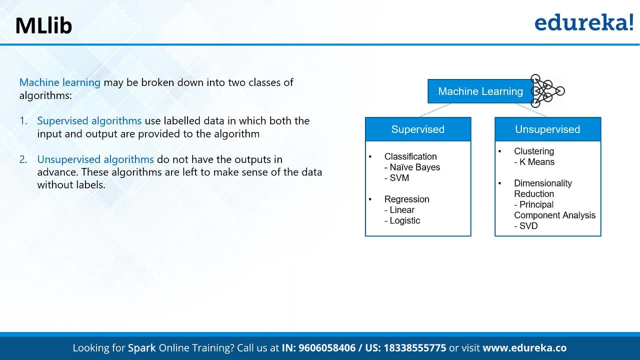 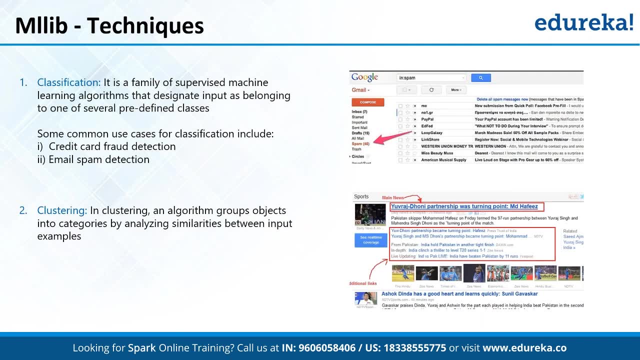 So all these types of algorithm can be implemented using spark right MLF techniques. I think it's like. this is like how the machine learning algorithms are implemented as an- you know, detecting the spam emails, or classification. That's nothing but like detecting the spam emails. 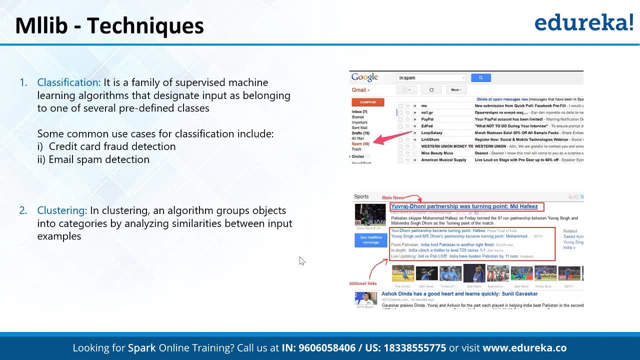 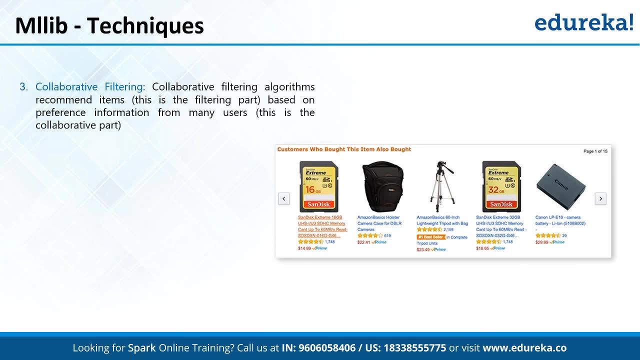 This is nothing but the example of classification right, Clustering as in, like you see, right, this, this newsfeed is. this newsfeed belongs to sports section or it belongs to politics, right? All these things? Collaborative filtering again, like whenever you purchase anything from the e-commerce portal. 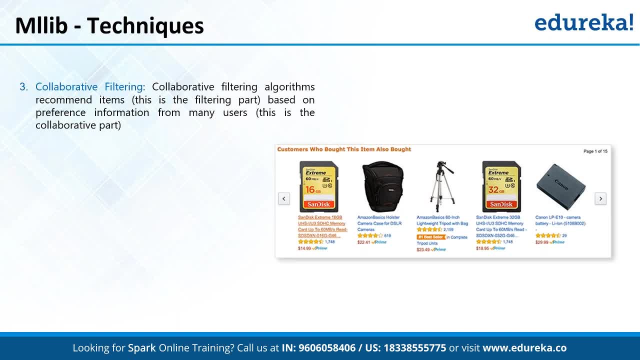 right. So whenever you purchase anything you will be getting, You will be getting this, basically recommendation right. So it will say, like customer who bought this item also bought this. So how is that happening? So all the e-commerce site they are storing, they have the history. 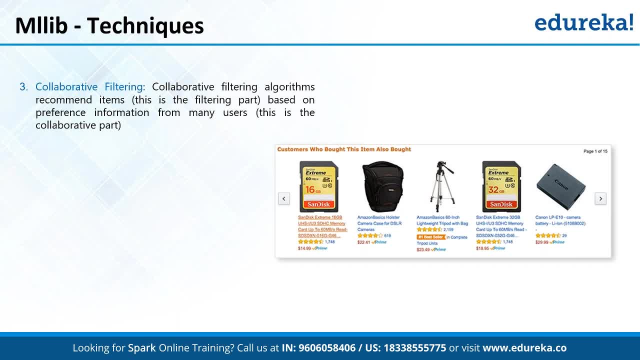 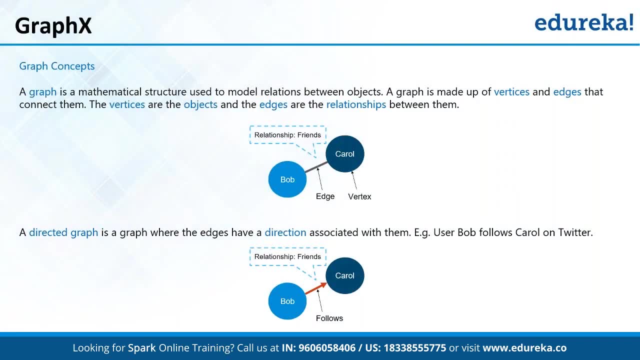 of your purchases and they are comparing that history with other purchases, like, and whenever the choice is matching, they will recommend that. Okay, graphics- It's like doing the analysis on the graph data. example. It's like we do have friends- of friends on Facebook. 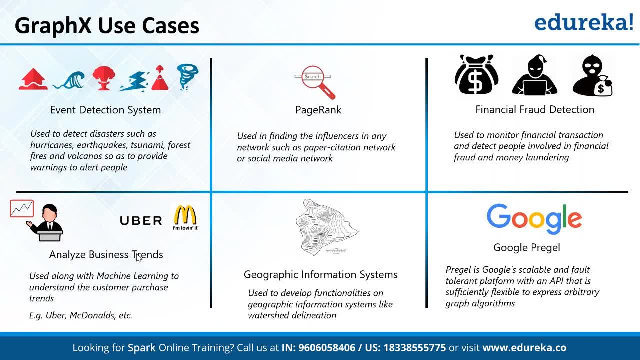 So, when it comes to graphics use cases, we do have, like Uber and McDonald's, doing the analysis to understand the customer purchase. Then we do have page rank algorithm, as in whenever you search anything on Google, right? So what? whenever you purchase anything on Google? 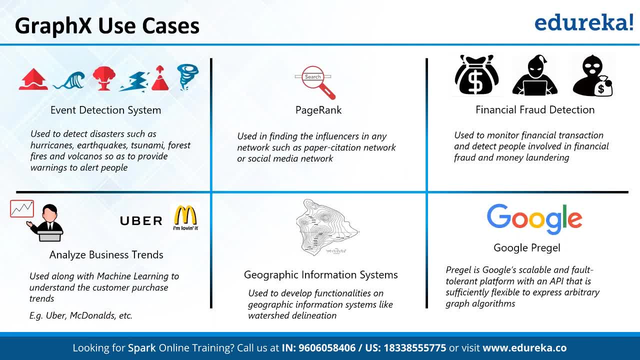 right What it will be doing. Sorry, whenever you search anything on Google, it will be showing some pages in the top and some pages the bottom. So how is that happening? that all is happening based on the page rank algorithm. Thank you, guys. Thank you, Thank you.